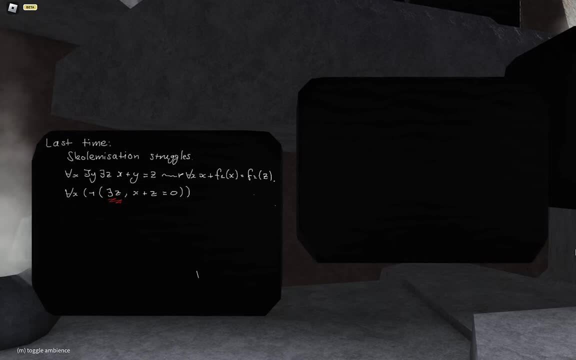 front, as far as I can, then that existential quantifier is going to turn into a universal quantifier, right? So you kind of have this question: what are the existential quantifiers, This one that I've underlined in red? is that an existential quantifier or is it a universal? 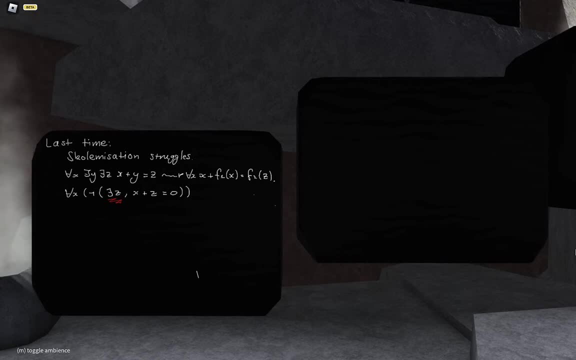 quantifier in disguise, right? Okay, so that was a very good observation that Billy made, And my counter was that it doesn't matter. and the reason why is because this spolimization, for the sake of the proof that I'm giving of the Axe-Greuthen-Deak Theorem, the spolimization 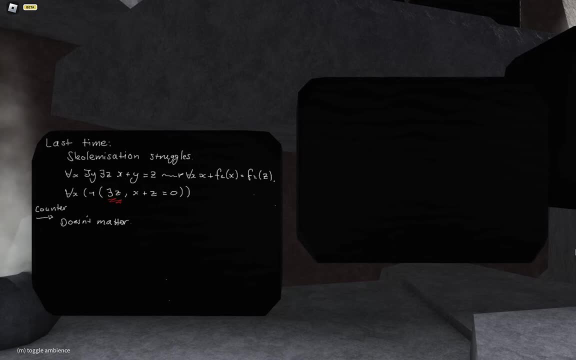 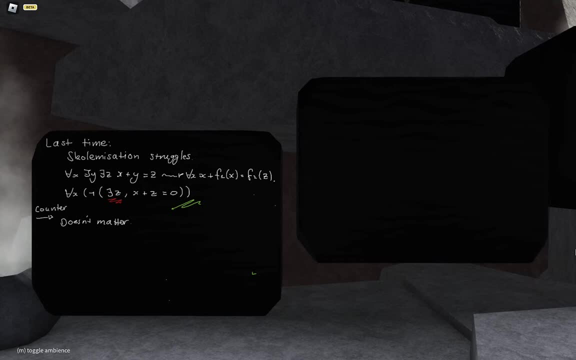 still holds. you can just decide that that is an existential quantifier and you can replace it with a column function symbol. you just might not end up with any formula that has any relationship to the previous one whatsoever, right? So that's a bit clumsy and that's a bit messy. 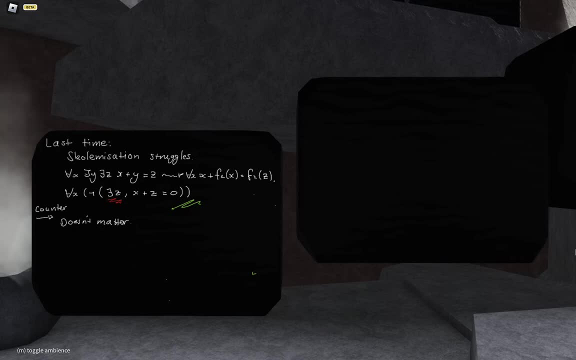 The way that we can make this a whole lot clearer is to introduce what's called the pre-next normal form of a first-order statement, And this is what the missing piece was last time. The pre-next normal form is a negation normal form and it has all of the quantifiers pulled. 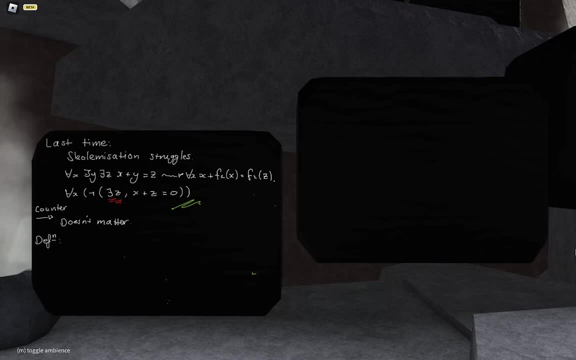 out the front. So let's define such a thing: A first-order formula, phi. In some first-order theory t is in pre-next normal form if phi is equal to quantifier 1, x1,, dot, dot, dot. quantifier n, xn, phi, prime, with phi prime quantifier-free. 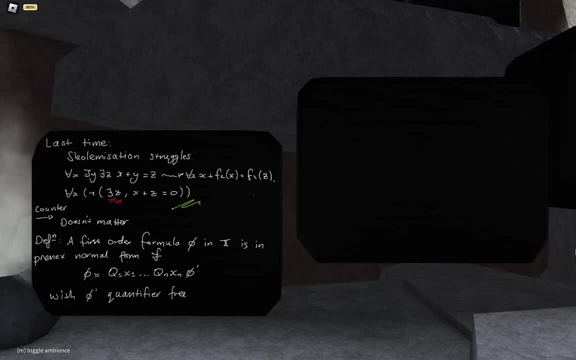 Okay, So qi is an element of for all and there exists. yeah, okay, And then as long as we only ever consider formulas that are inside pre-next normal form, then this question doesn't arise. So to put it explicitly, this second first-order formula that I wrote down is not in pre-next. 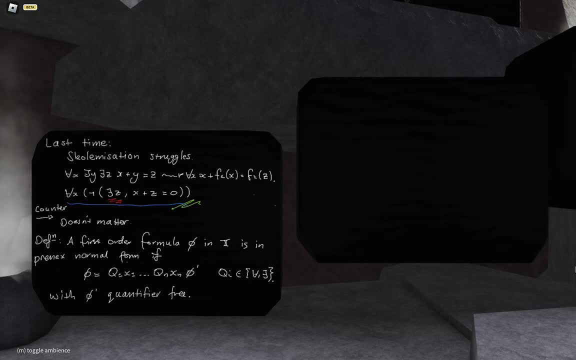 normal form. So you get this kind of confusion. Okay, So the first one is in pre-next normal form, because it's very explicit. This is the extension quantifiers that I wish to replace and in such a situation I do get equivalence between the original first-order formula and the spellimization of the formula. 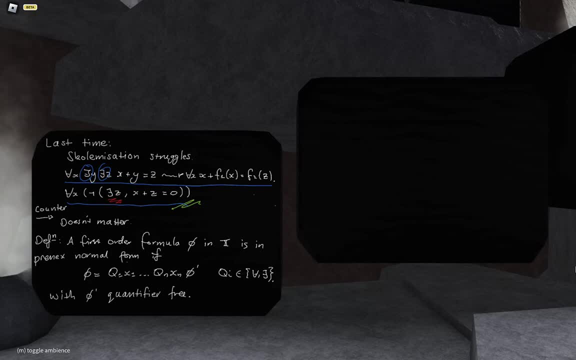 Okay, And the proposition which I'm going to use is that every first-order formula is going to have an associated pre-next normal form which is equivalent in quite a strong sense. So you can prove the spellimization from sorry, you can prove the pre-next normal form. 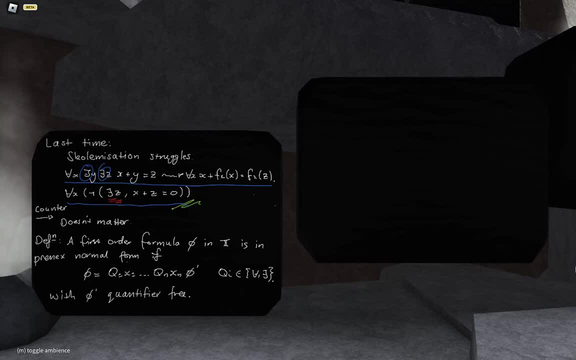 associated to a first-order theory, from- sorry, associated to a first-order formula, from the theory that that formula was defined over and that first-order formula that you started off with, And vice versa. So I can write down, I can write down that proposition and for this seminar we will. 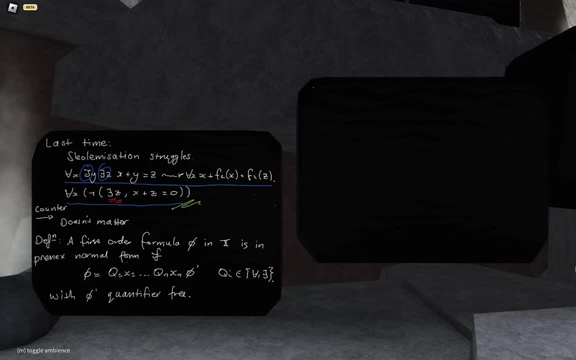 be just taking this for granted Proposition. Prefer every first-order formula phi. Now, everything tends to operate. That's theằngisha. So was arranged graphically in some very useful ways And let's see, We have some first-order theory. two with t. 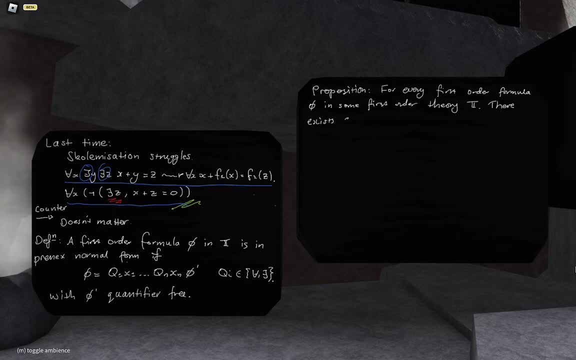 There exists a pre-next normal for phi such that t is null, And I'm making it to match Waldron And we'd love to use that in order to follow along. We don't have the broth here. Bye, have a great day everyone. 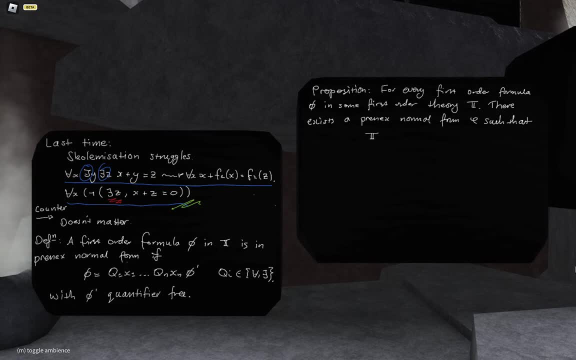 t union phi can prove var phi or phi and t union phi can prove phi. cool, okay. and then, in this first order, theory is where all of the formulas are in pre-next normal form which we're going to be concerning ourselves with. okay, so now let's try to uh head towards the lower lohenheim's golem theorem, the lower. 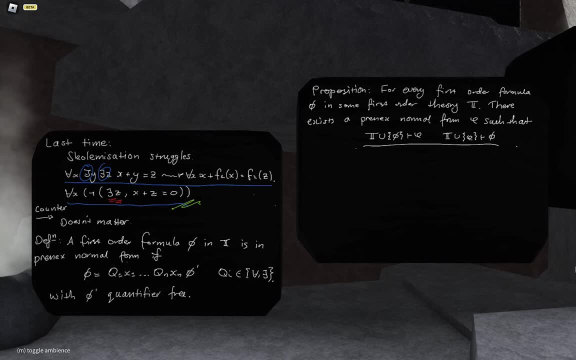 lohenheim's golem theorem is a statement that if you have a model for some first order theory, then if that model is an infinite cardinality, then you can also construct a model of the same first order theory, but of any cardinality less than the cardinality of the original model. there are a couple of more uh hypotheses that you 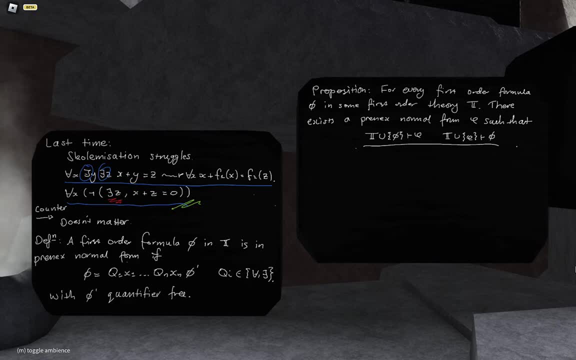 need. but these are just hypotheses upon the first order formula um that make the scholomization satisfy this proposition right, um. so i'm just going to be assuming that we are dealing with first order theories where all of the formulas are in pre-next normal form. 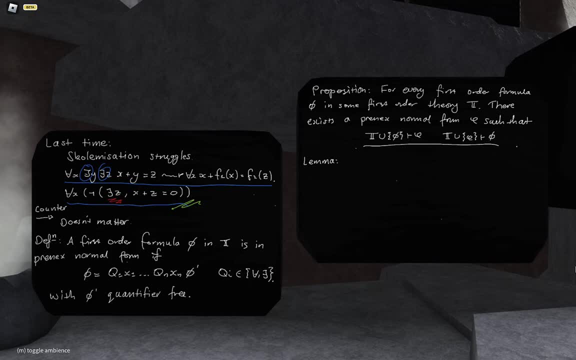 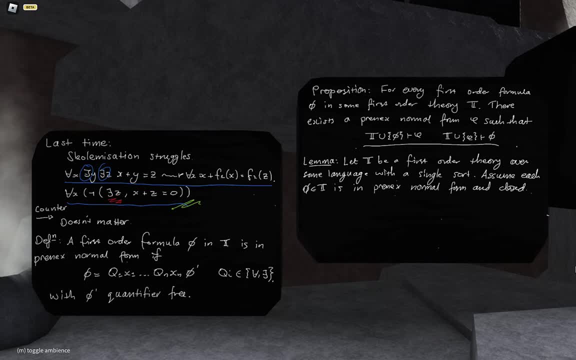 they just mean that the formulas have no free variables. so the favorable set is the, the favorable set is the empty set. and the statement is: if t admits a model. and the statement is: if t admits a model, then so does the spolimization. oops, then so does the spolimization of the model. 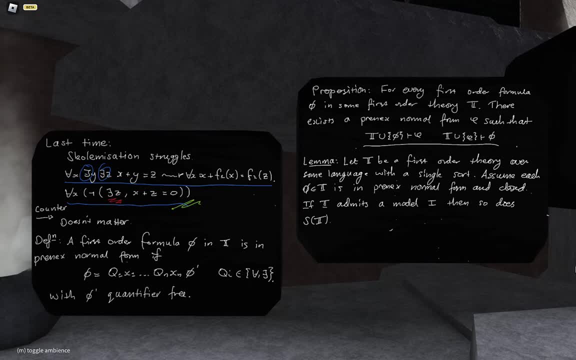 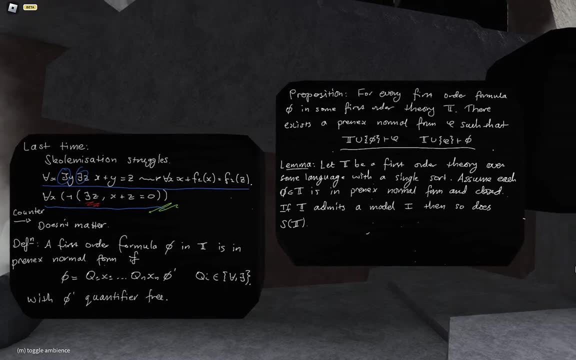 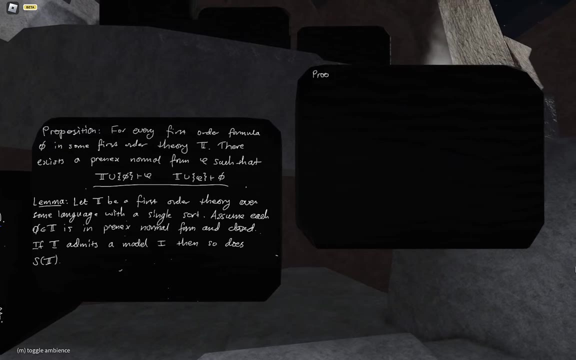 then so does the spolimization of t. okay, now let me prove this. okay, i'm going to need to talk about the. okay, i'm going to need to talk about the number of uh variables inside fire, which are. number of uh variables inside fire, which are: 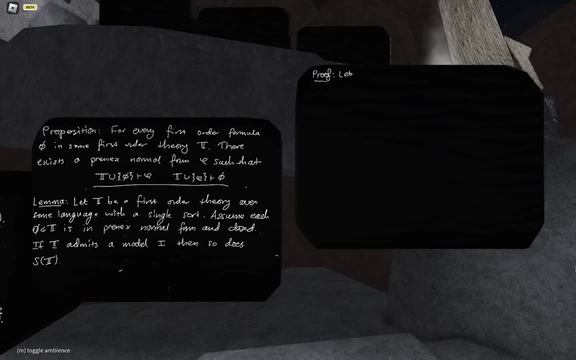 specifically by an existential quantifier. so i'll let this specifically by an existential quantifier, so i'll let this integer be denoted m. integer be denoted m. integer be denoted m. okay, and the technique okay, and the technique okay and the technique it's. it's a proof by induction of sorts. 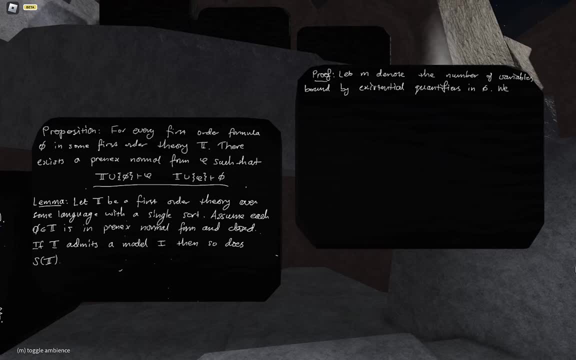 it's, it's a proof by induction of sorts. it's, it's a proof by induction of sorts, but i'm inducting on a, but i'm inducting on a, but i'm inducting on a finite quantity. so, really, what i'm showing, 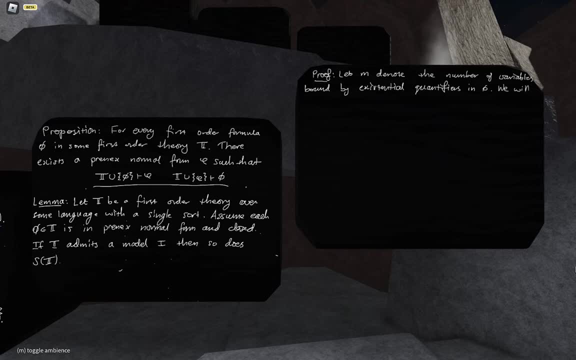 finite quantity. so really what i'm showing, finite quantity. so really what i'm showing is: for any, for any, for any, i equals one up to m minus one. i equals one up to m minus one. i equals one up to m minus one if there is a model. 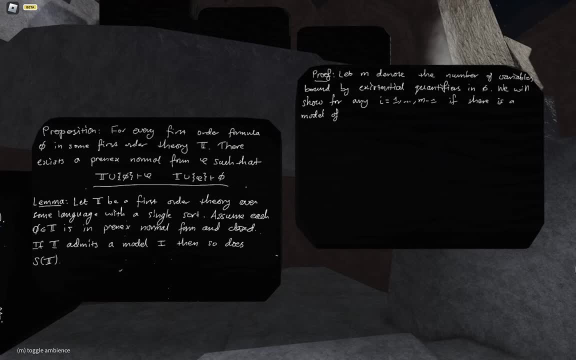 there is a model, there is a model, a model i, such that the interpretation of the ith scalamization is equal to one, of the ith scalamization is equal to one, of the ith scalamization is equal to one, then then, then there is also a model of the i plus one. 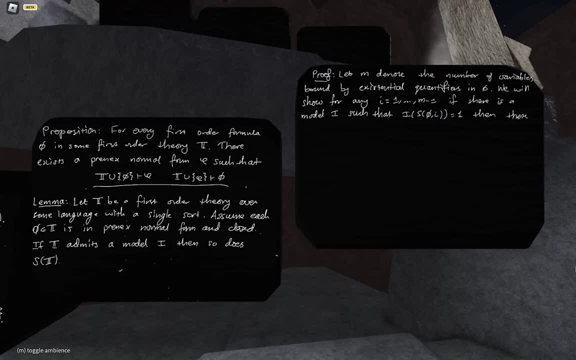 there is also a model of the i plus one. there is also a model of the i plus one for scalamization, for scalamization, for scalamization. sorry, what is the formula phi from is sorry. what is the formula phi from is sorry. what is the formula phi from? is this just any formula at all, or is it? 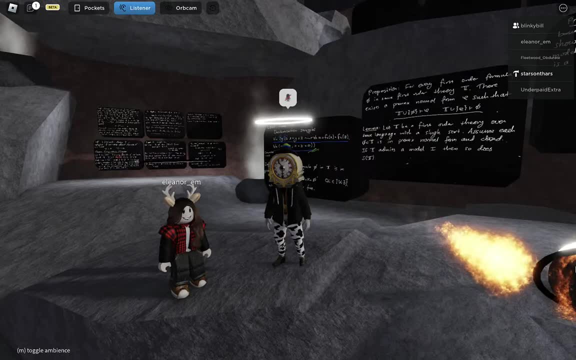 this just any formula at all? or is it this just any formula at all? or is it like, like, like? this is true in the. this is true in the. this is true in the: uh, this is one of the formulas that are: uh, this is one of the formulas that are. 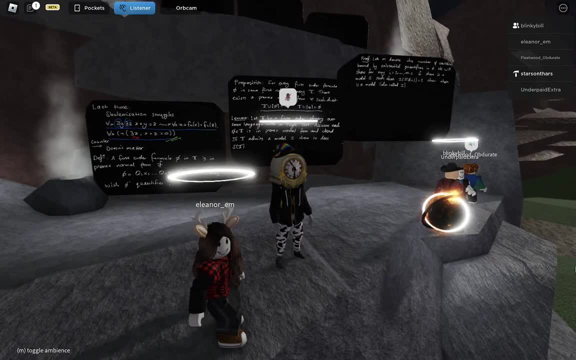 uh, this is one of the formulas that are inside the first order theory t, inside the first order theory t, inside the first order theory t that satisfies the hypotheses inside the. that satisfies the hypotheses inside the. that satisfies the hypotheses inside the lemma, lemma, lemma. so i thought that i put: 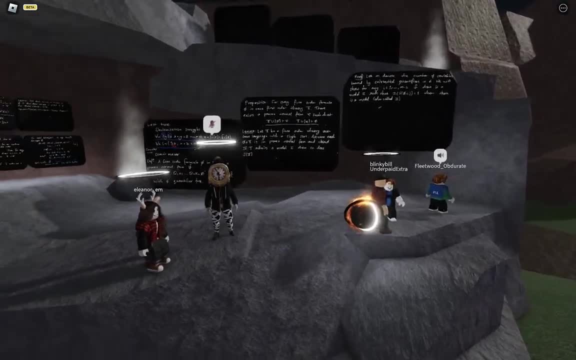 so i thought that i put. so i thought that i put fi in the statement, fi in the statement, fi in the statement. should i not do that? should i not do that? should i not do that? yeah, yeah, you did, i'll just check. yeah, yeah, you did, i'll just check. 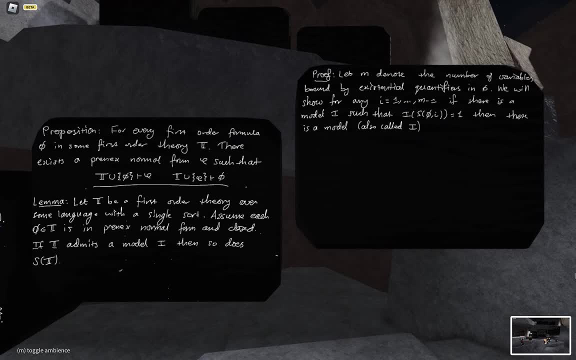 yeah, yeah, you did, i'll just check. okay, cool, so so you're doing uh. so, so you're doing uh. so so you're doing uh, you're proving something about each phi. you're proving something about each phi. you're proving something about each phi. yeah, okay, and this is the statement that i'm. 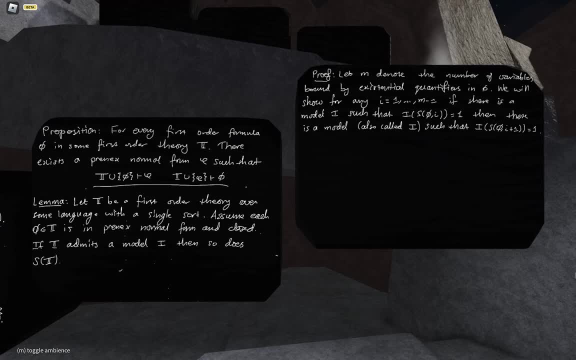 okay, and this is the statement that i'm okay, and this is the statement that i'm proving that, proving that, proving that if i have this interpretation, that if i have this interpretation, that if i have this interpretation that interprets the ice polarization as one, interprets the ice polarization as one, 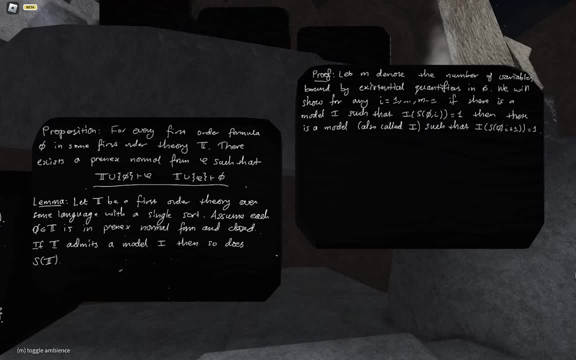 interprets the ice polarization as one, then then, then i can, i can. what i'm going to do is i'm going to. what i'm going to do is i'm going to. what i'm going to do is i'm going to extend, i extend, i. 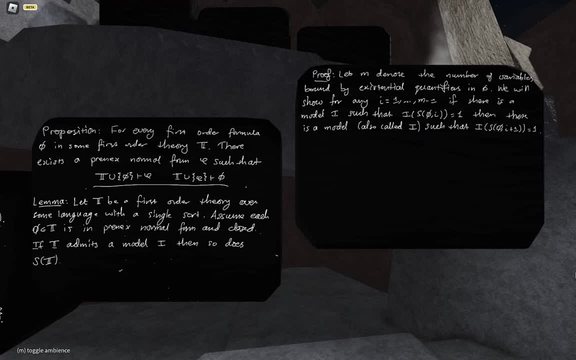 extend i to yeah. an interpretation that interprets to yeah. an interpretation that interprets to yeah. an interpretation that interprets: the i plus one, the i plus one, the i plus one column function in such a way where the column function in such a way where the 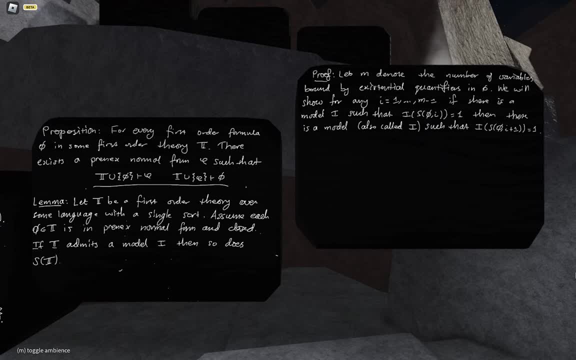 column function in such a way where the interpretation is definitely equal to one. interpretation is definitely equal to one. interpretation is definitely equal to one of the i plus one of the i plus one of the i plus one. colonization, colonization, colonization, okay, okay, okay. is there a reason that it's so called i? 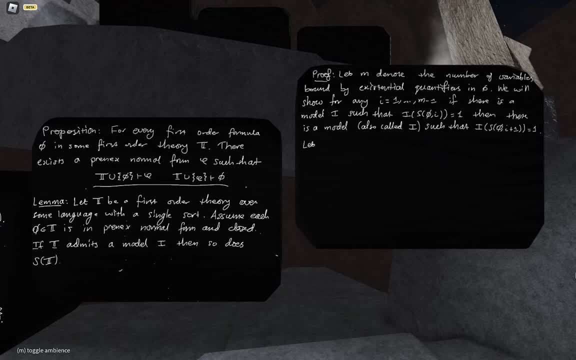 the, the, the interpretation, or the index interpretation, or the index interpretation or the index, the interpretation. you said also the interpretation. you said also the interpretation. you said also: called i in brackets, called i in brackets, called i in brackets. oh, because i'm extending, i, so i. oh, because i'm extending i, so i. 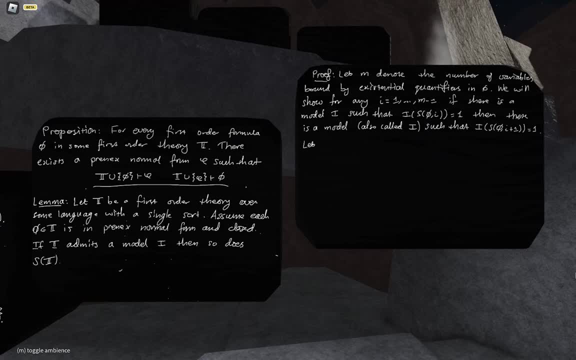 oh, because i'm extending, i, so i is an interpretation and what that means is an interpretation, and what that means is an interpretation. and what that means is that we have an assignment of a. is that we have an assignment of a, is that we have an assignment of a function to every function symbol. we 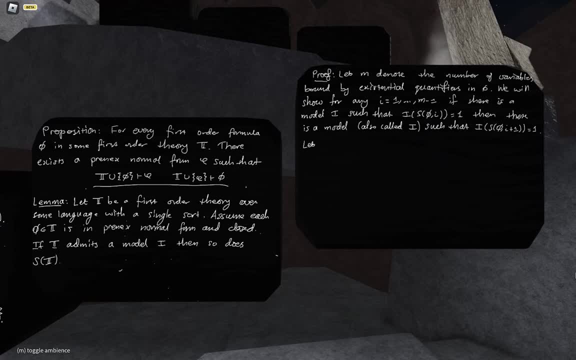 function to every function symbol. we function to every function symbol. we have an assignment of a relation to have an assignment of a relation, to have an assignment of a relation to every relation symbol, etc. and every relation symbol, etc. and every relation symbol, etc. and all that i'm going to end up doing is 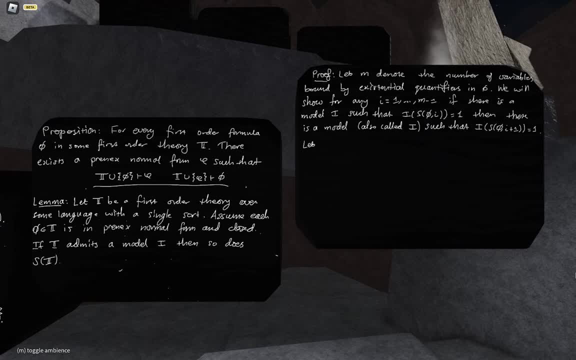 all that i'm going to end up doing is all that i'm going to end up doing is extending i to also interpret the i plus. extending i to also interpret the i plus. extending i to also interpret the i plus once column function, which does not once column function, which does not. 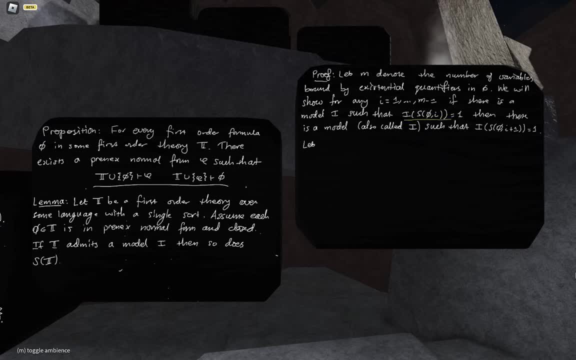 once column function which does not appear, appear. appear inside s of phi, i right. so i'm just inside s of phi, i right. so i'm just inside s of phi, i right. so i'm just lazily calling it. i because it's an lazily calling it, i because it's an. 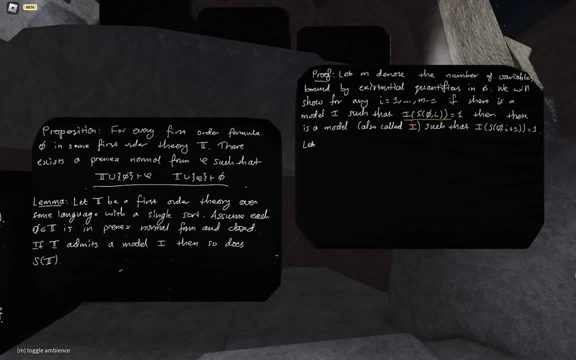 lazily calling it i because it's an extension, extension. extension. in reality. call that j. in reality. call that j. in reality. call that j. and identify. you know, just observe. you can observe afterwards that as an. you can observe afterwards that as an. you can observe afterwards that as an extension, j. 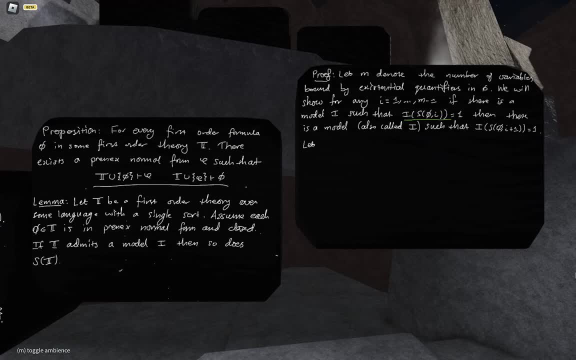 extension j, extension, j. okay. so all i'm going to do is take. okay. so all i'm going to do is take. okay. so all i'm going to do is take the leftmost existential quantifier, the leftmost existential quantifier, the leftmost existential quantifier, and replace that with a column function. 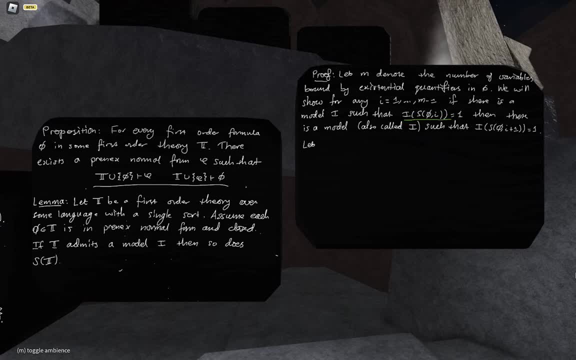 and replace that with a column function, and replace that with a column function and observe how the interpretation flows and observe how the interpretation flows and observe how the interpretation flows through, through, through that substitution. it's actually a that substitution. it's actually a that substitution. it's actually a pretty simple proof once you look at it. 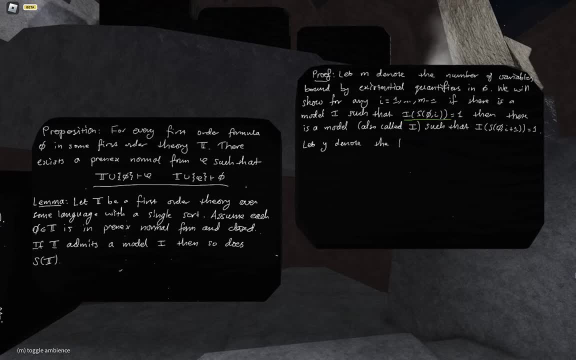 pretty simple proof once you look at it. pretty simple proof once you look at it. so let y so, let y so, let y deny. so let y deny. leftmost existentially bound quantifier. leftmost existentially bound quantifier. leftmost existentially bound quantifier in phi. 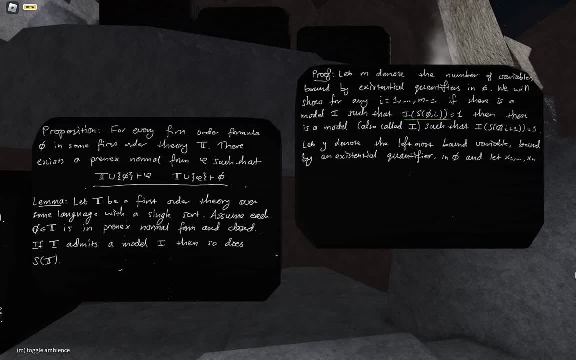 in phi, in phi, and and. and. let x1 up to xn be. let x1 up to xn be. let x1 up to xn be. those variables inside phi that are bound. those variables inside phi that are bound. those variables inside phi that are bound by universal quantifiers that occur to 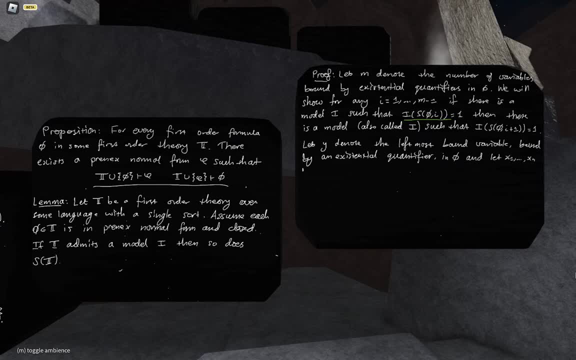 by universal quantifiers that occur to, by universal quantifiers that occur to the left of the left of the left of y. do you mean an existential quantifier in? do you mean an existential quantifier in? do you mean an existential quantifier in phi or in s phi i? 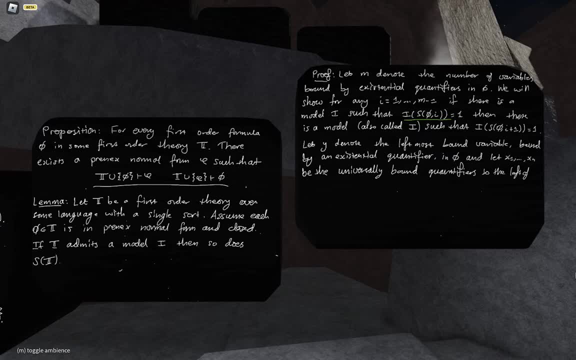 phi or in s phi. i phi or in s phi i. oh, that's a good question. oh, that's a good question. oh, that's a good question. i do mean s phi. i thank you. i do mean s phi, i thank you. should i get that wrong in the notes? 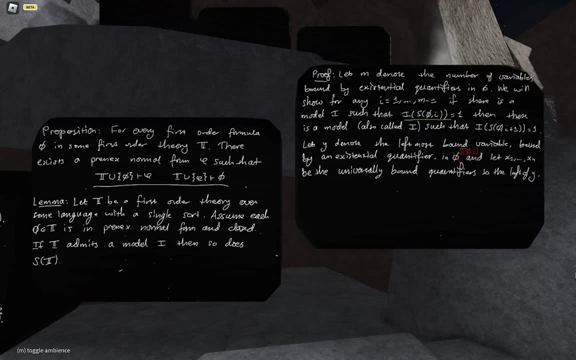 should i get that wrong in the notes? should i get that wrong in the notes? yep, yep, yep. okay, good pickup, thanks. oh yeah, that flows through. oh yeah, that flows through. oh yeah, that flows through. okay, that's fine, we can adapt so s. okay, that's fine, we can adapt, so s. 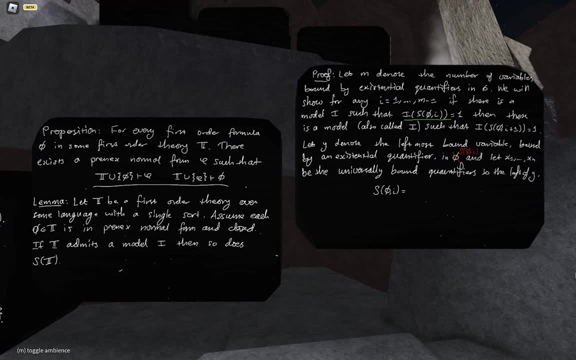 okay, that's fine, we can adapt. so s phi, i phi, i phi, i keep in mind, phi, keep in mind, phi, keep in mind. phi is in pre-next normal form, so all of is in pre-next normal form. so all of is in pre-next normal form, so all of the quantifiers are at the front. so s phi. 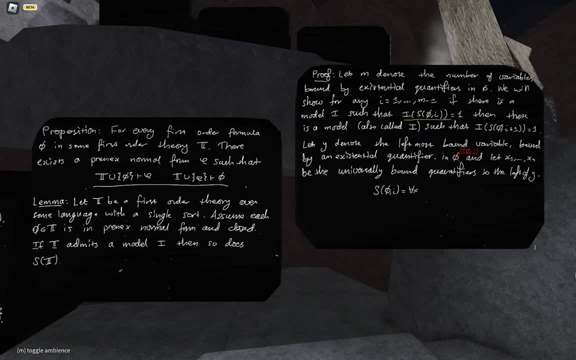 the quantifiers are at the front. so s phi, the quantifiers are at the front. so s phi, i, we can write out, i, we can write out, i, we can write out pretty easily. it's pretty easily, it's pretty easily. it's a whole stack of universal quantifiers. 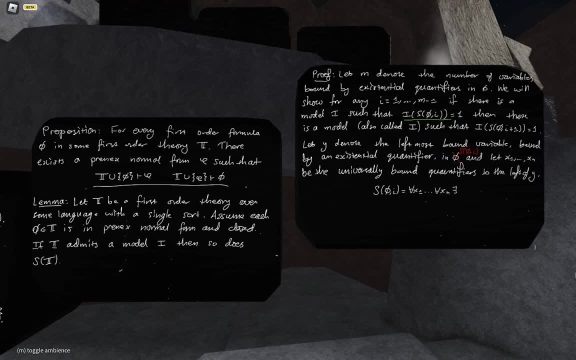 a whole stack of universal quantifiers, a whole stack of universal quantifiers, and we know that there's n of them, and we know that there's n of them, and we know that there's n of them by definition of n, and then by definition of n, and then. 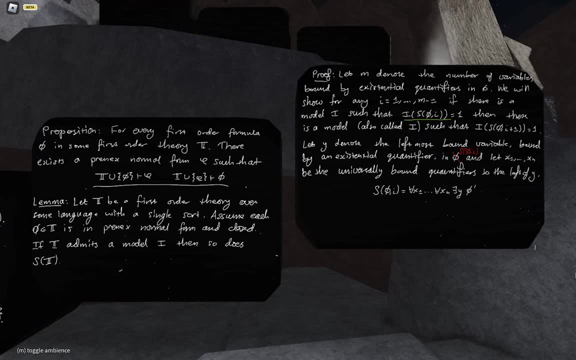 by definition of n, and then there is the existential quantifier y, there is the existential quantifier y, there is the existential quantifier y, followed by phi prime, and we just have followed by phi prime, and we just have followed by phi prime, and we just have no assumption on phi prime, right? so 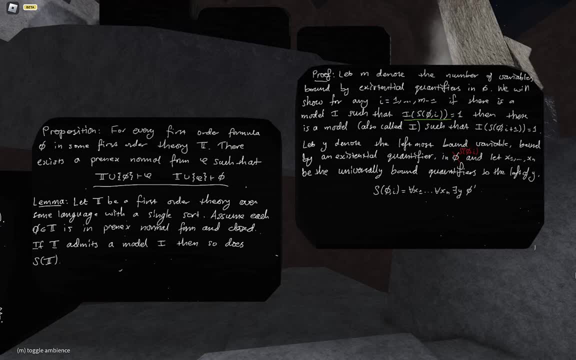 no assumption on phi prime right. so no assumption on phi prime right. so phi prime may or may not have quantifiers. okay, okay, okay, but. but but that's helpful, because now that's helpful, because now that's helpful because now i can relate the i and the i plus one. 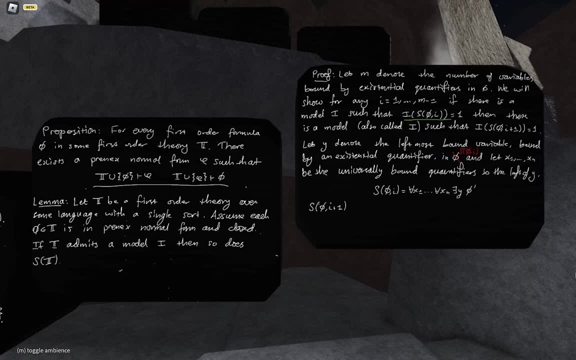 i can relate the i and the i plus one. i can relate the i and the i plus one specialization. we notice that the i plus specialization. we notice that the i plus specialization. we notice that the i plus one specialization. one specialization is equal to s of the formula for all. 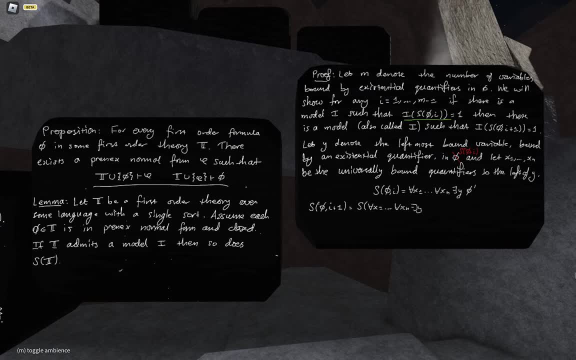 is equal to s of the formula for all, is equal to s of the formula for all: x1 dot dot dot for all x, and there x1 dot dot dot for all x, and there x1 dot dot dot for all x. and there exists y, exists y. 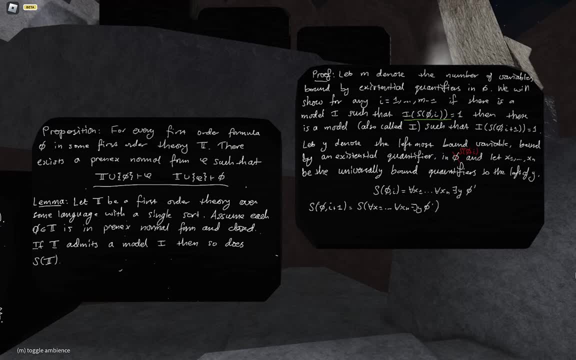 exists. y phi prime. i haven't done anything phi prime. i haven't done anything phi prime. i haven't done anything complicated in that step, whatsoever. complicated in that step, whatsoever, complicated in that step, whatsoever. that's just the previous line, that's just the previous line, that's just the previous line, that's i plus one, and then that's. 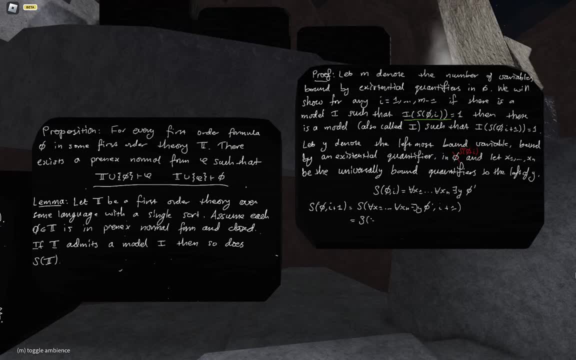 that's i plus one, and then that's that's i plus one, and then that's equal to equal to equal to the, the the ith columnization of phi prime. but i'm going to do the of phi prime, but i'm going to do the of phi prime, but i'm going to do the substitution. 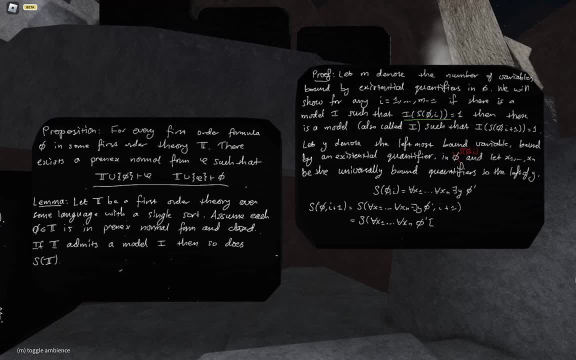 substitution. substitution of y for this for the i plus one of y for this for the i plus one of y for this for the i plus one column function manually. so i just put column function manually. so i just put column function manually. so i just put here y. 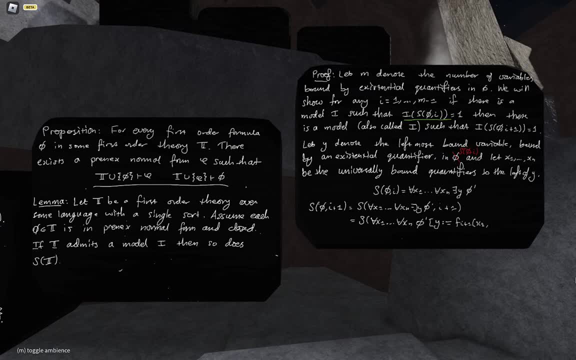 here y, here y substituted f. i plus one substituted f. i plus one substituted f. i plus one of x, one of x, one of x, one up to x, n. up to x, n. up to x, n. square bracket, square bracket. square bracket. comma, comma. comma i i. 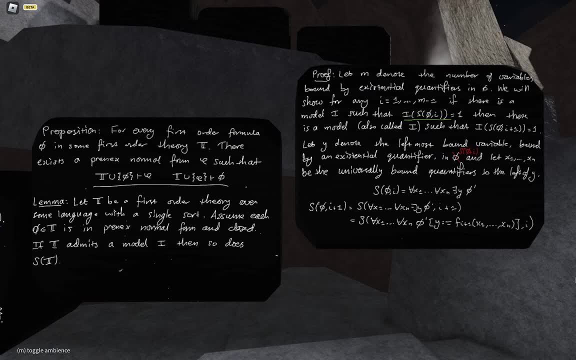 i close bracket. close bracket. close bracket. right, right, right, okay, okay, okay. and then i'm going to use the fact that, and then i'm going to use the fact that, and then i'm going to use the fact that i have a. i have a, i have a model of this in order to define. 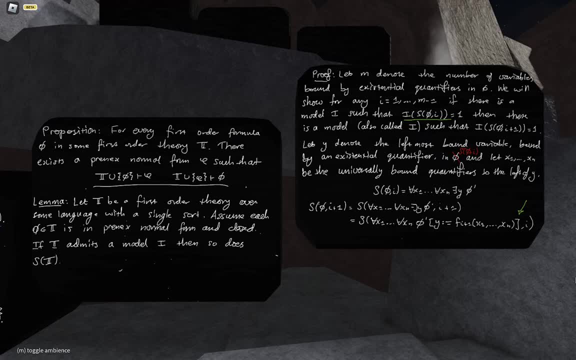 model of this in order to define model of this, in order to define a function which i'm going to interpret, a function which i'm going to interpret, a function which i'm going to interpret the i plus one function symbol as: the i plus one function symbol as: 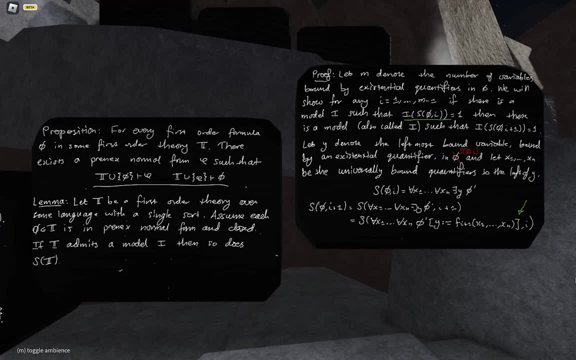 the i plus one function symbol as okay, okay, okay, so i need to move to the next board. so i need to move to the next board. so i need to move to the next board. and do we do platforming for that i? and do we do platforming for that i? 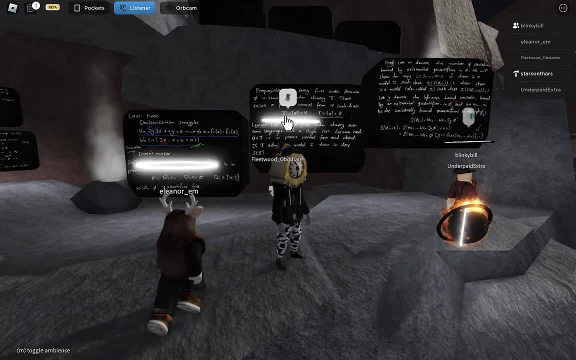 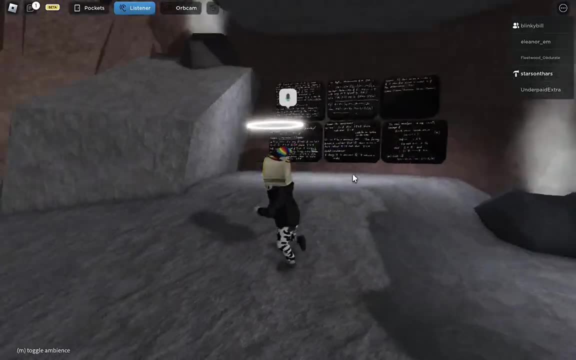 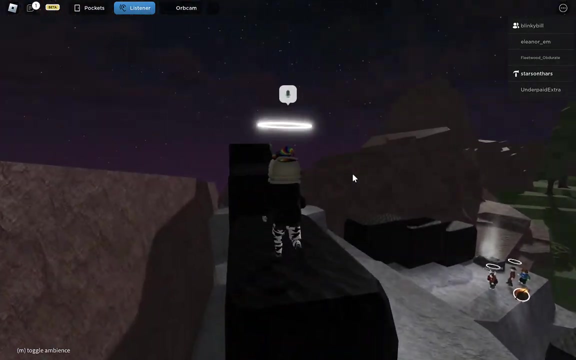 and do we do platforming for that? i think we do. you can also walk around another way. you can also walk around another way. you can also walk around another way. okay, everyone finds their own way. everyone finds their own way. everyone finds their own way. i don't. i got two characters to do so. 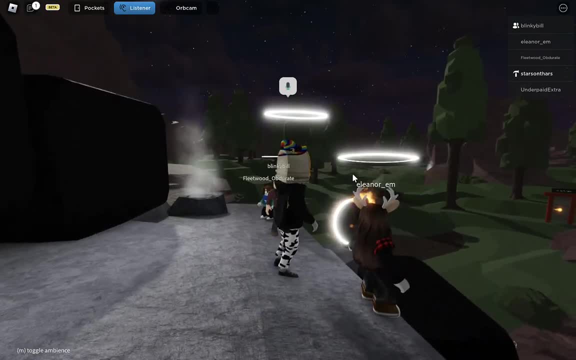 i don't, i got two characters to do so. i don't, i got two characters to do so. give me a second, give me a second, give me a second. oh my god, it's better to walk on the vents if you. it's better to walk on the vents if you. 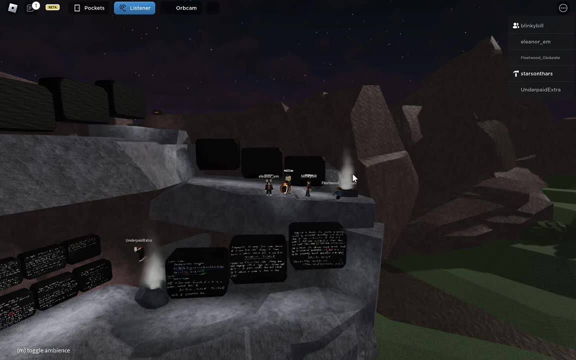 it's better to walk on the vents. if you jump on them, you don't go as high. jump on them, you don't go as high. jump on them, you don't go as high. really, really, really, i'm having, i'm having, i'm having the opposite experience right now. 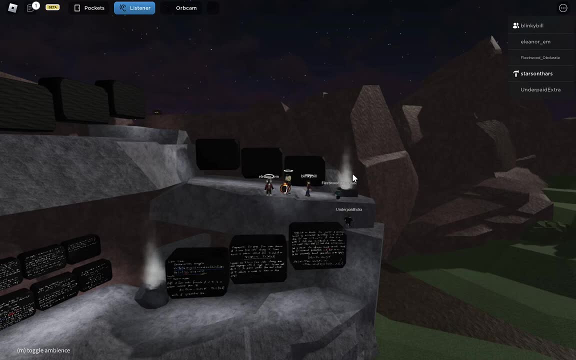 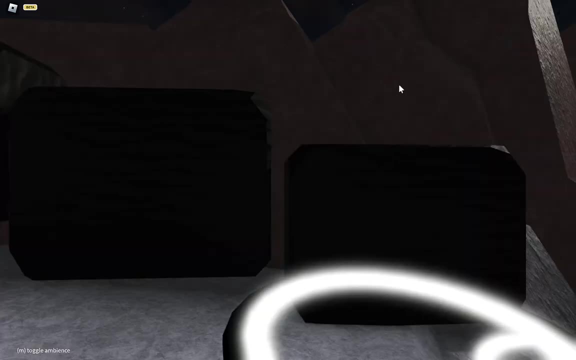 okay, there we go, okay, there we go. okay, there we go. we already, we already. we already established that i have no humility established that i have no humility, established that i have no humility down, okay, okay, okay, okay, okay, okay, we've got, we've got. uh, halos in the old. 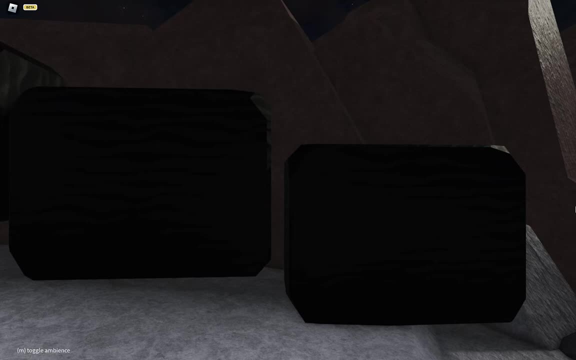 we've got. we've got uh halos in the old. we've got. we've got uh halos in the old cam, cam, cam. it's all good now i don't, i don't have a. it's all good, now i don't, i don't have a. 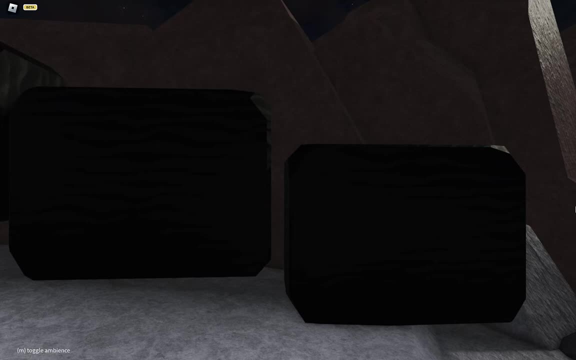 it's all good, now i don't. i don't have a halo that doesn't pertain to me. halo that doesn't pertain to me. halo that doesn't pertain to me, okay, okay, okay. so we'll define f uh. we'll define f uh. 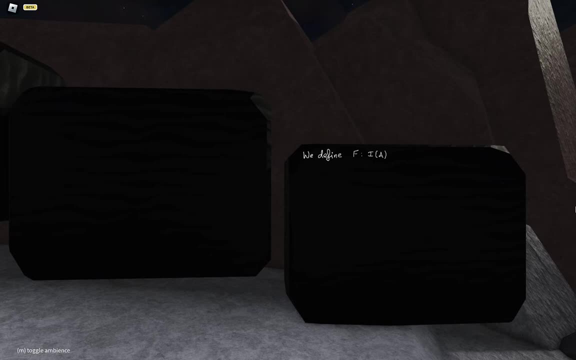 we'll define f. uh, oh, i guess i should say what a is so a. oh, i guess i should say what a is so a. oh, i guess i should say what a is so a is just going to be the one and only is just going to be the one, and only. 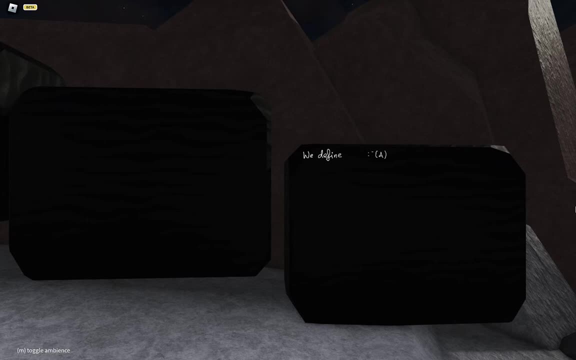 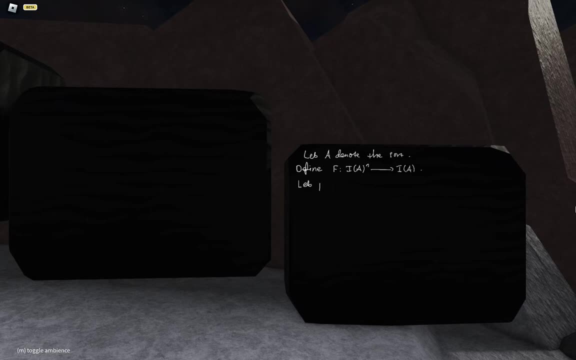 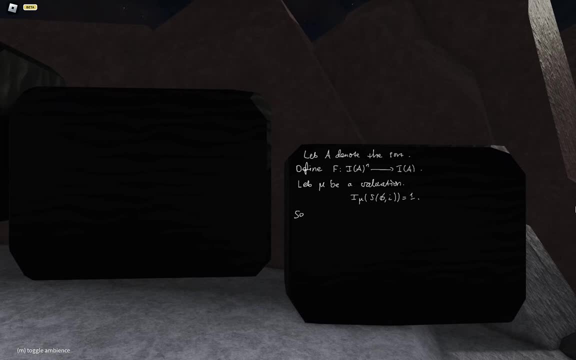 as of s phi, as of s phi i i. i is equal to one, is equal to one, is equal to one, and so this means that, and so this means that, and so this means that. oh, i mean useful, oh, i mean useful, oh, i mean useful. that means that, for all. 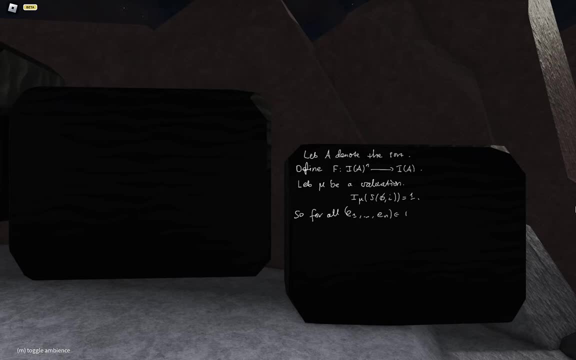 that means that, for all that means that, for all, a, all tuples of elements, a, all tuples of elements, a, all tuples of elements inside i, inside i, inside i of a to the n of a, to the n of a, to the n, there exists, there exists, there exists, e in i of a. 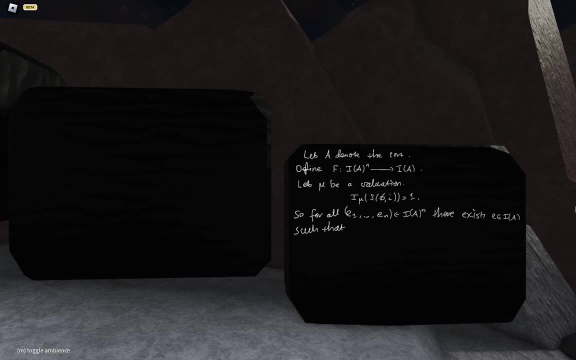 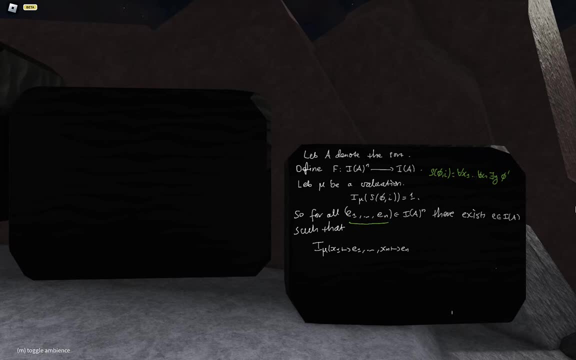 finished it. oh yeah, i did leave it out, so i haven't accounted for the. e is going to be some element where, if i interpret y as that element, then i get, uh, the evaluation mapping, for one right. we know that such a thing exists because we have a model of the arts column. 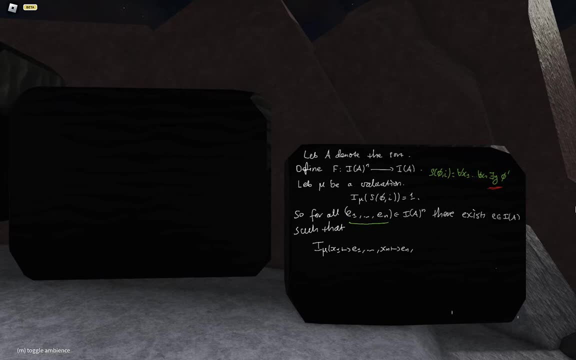 um, right, so you're not saying that he's. he's not the tuple e1 up to en. no, sorry, it'll make more sense once i've written my thing right. so don't forget that the arts colonization was this thing and we know that we have a model for that. and so for every e1 up to en, if i do these, 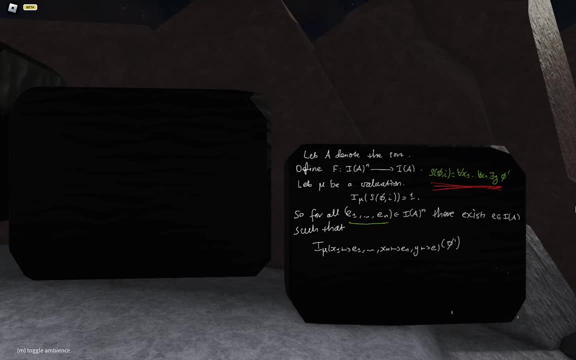 substitutions. there exists some y, sorry, some e, especially if y gets interpreted as e, then this entire thing maps to one right and so, uh, this is the point. this is the exact point in the proof. this comment's mainly for billy um, where last time you were asking if this entire thing is equivalent to choice in some. 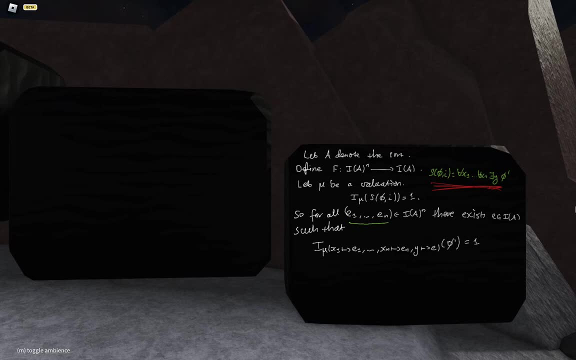 way right, because we remark at this point that there's not necessarily a unique e, right? so what i need to do is making choice of e for all such tuples. i'm doing that in the meta theory, right? so i'm doing that in the meta theory right? so i'm doing that in the meta theory. 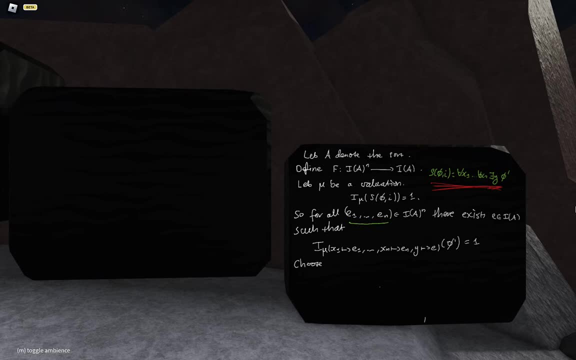 right. so, dan, you also made a comment about this last time, so i'm using choice in the meta theory here. choose an e for all such e1 up to en, and then i'm going to define f from i of a, n to i of a, as e1. dot, dot, dot e n maps to. 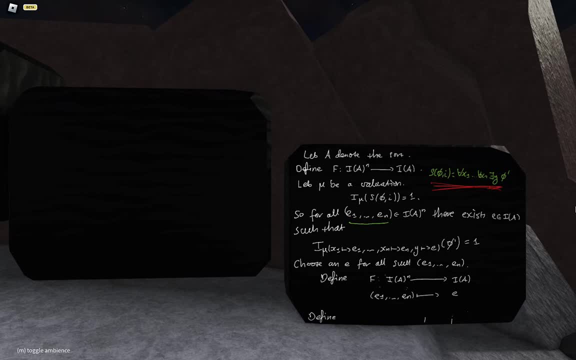 to that E, and then I define the interpretation of F- I plus one- as this F right, And then I've clearly extended the model out to the I plus one for scolomization. you know the first order theory pertaining to that. 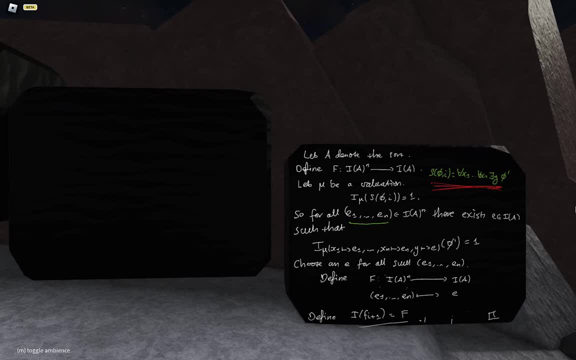 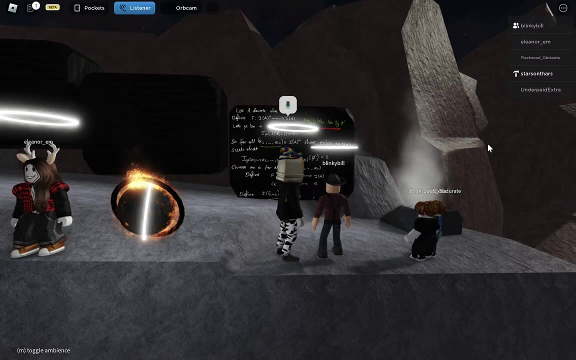 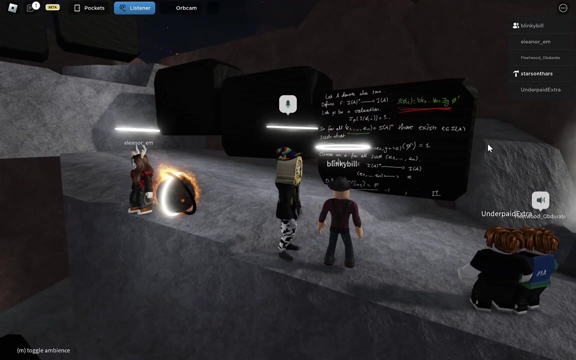 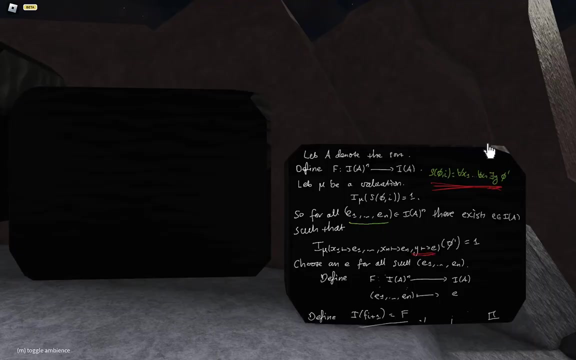 So that's an interesting step. Does anybody have any comments about that? Yeah, I mean, I feel that. can you put that in some words, though? Do you want me to say it again? You see, we don't know that this E is unique. 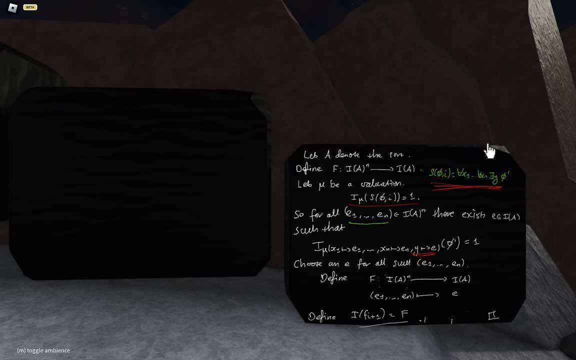 but we know that it exists. because of this, We know that we have some interpretation that sets this equal to one, And what that interpretation says is that, when you get to this existential quantifier, there has to be some element inside the domain. essentially, if I set Y to be equal to that element, 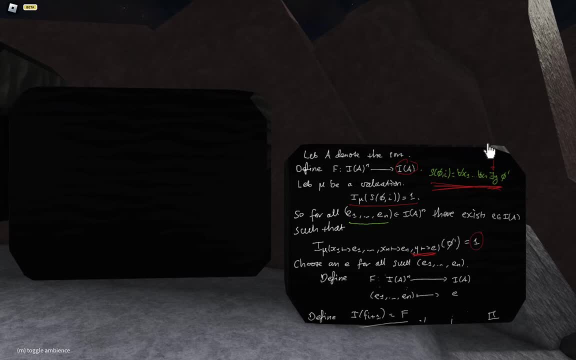 and then I carry on with my interpretation. I eventually get down to the value one. right Now, the interpretation doesn't have an element E in its hands, but I, as a data theory, am saying there is such an E out there somewhere. 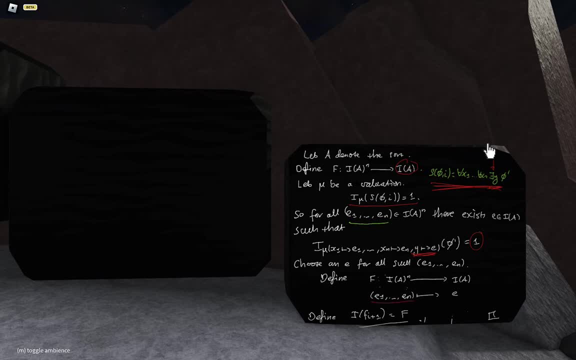 Make a choice of such an E, for you know this E right H, tuple E1 up to EN and then use that to define a function right. So the interesting question is, what have I used in the meta theory to do that? 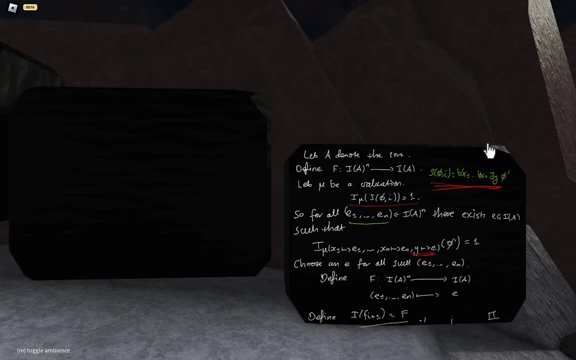 And I believe the statement is like it might even be strong choice right. So I've got some pretty heavy hammers inside the meta theory at this point. Where are you Will? It seems like there's a wind in your microphone or something. 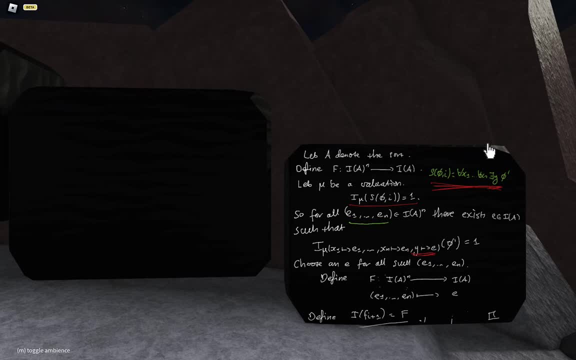 Oh dammit, yeah, you caught me. I'm outside. Do I need to? Is it really bad Or is it okay? Just now it was it's sort of noticeable in general but it's not so bad, but just then it was pretty severe. 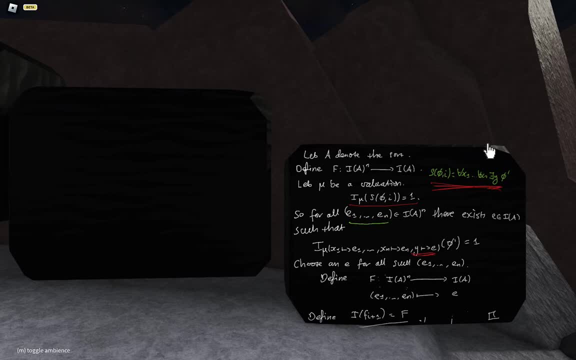 I don't have a good place at the uni to make a lot of noise. I okay, do tell me if it gets really bad and I'll jump inside. I think I can see a spot, but I'll try to persevere with this for now. 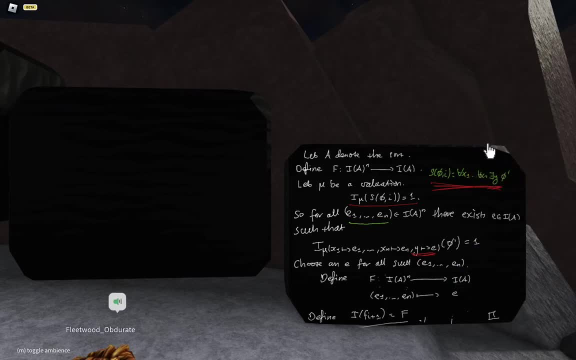 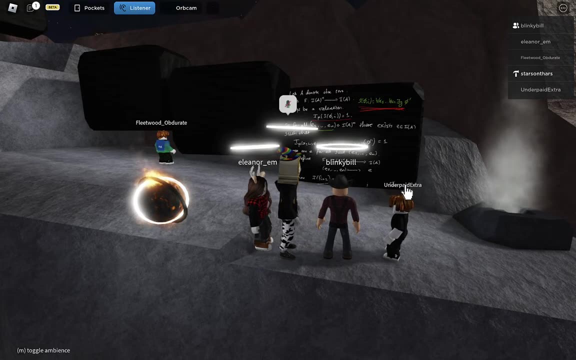 Sure, Yeah, I don't have any sensible grounds for complaint about the choice business. I'll just stew on it quietly. Yeah, yeah, I thought you were a fan of choice. I'm a fan of choice when it's an axiom. 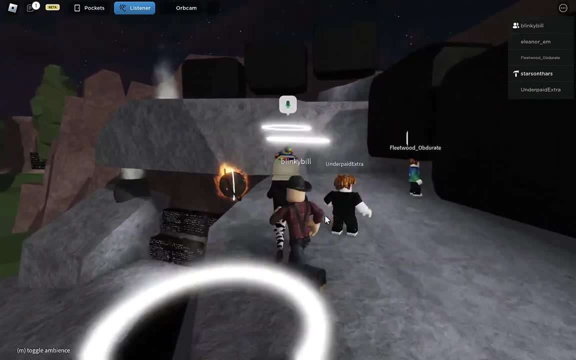 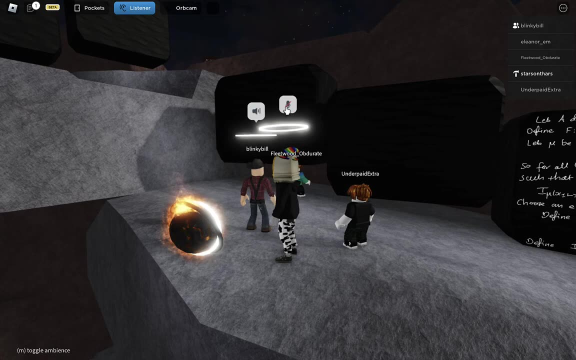 not some voodoo, that happens in the meta theory. but okay, Yeah, I agree with Dan. An axiom of the meta theory: when you're just doing normal mathematics here, It's just: it's turtles all the way down. That's what I just heard. 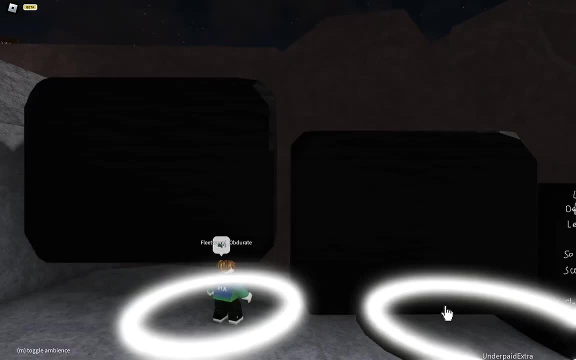 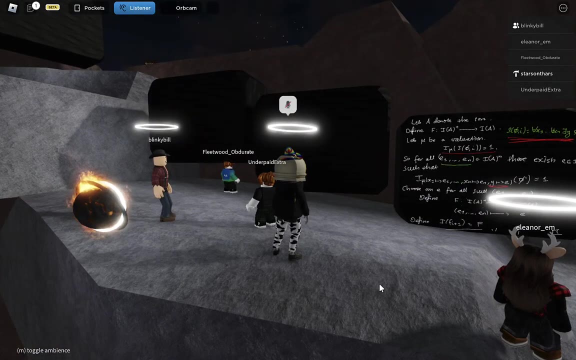 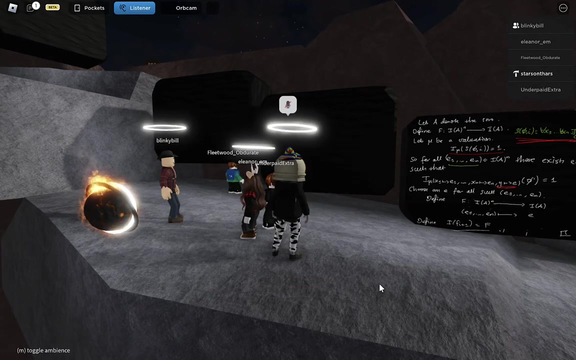 Yeah, The. the one thing that I would tell you on, Dan, though, is when we were doing the lecture on models, I was talking about all this hoo-ha of the Platonistic existence of objects and math out there, et cetera. 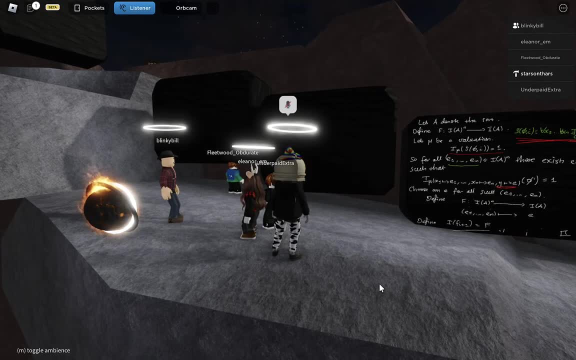 And you kind of refuted that by saying all that you're doing with these models is reinterpreting first-order theories in other first-order theories. So my understanding is you're essentially just you know you are reinterpreting them and you are reinterpreting them. 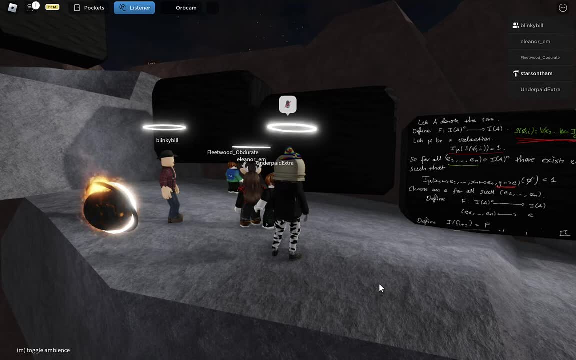 essentially just taking everything that happens inside a model is happening inside the first order theory of zf or zfc or zfcu, whichever one you kind of pick to take right. so if you just go ahead and take zfc, then i've just used the axiom choice inside zfc there, yeah, i'm totally fine with. 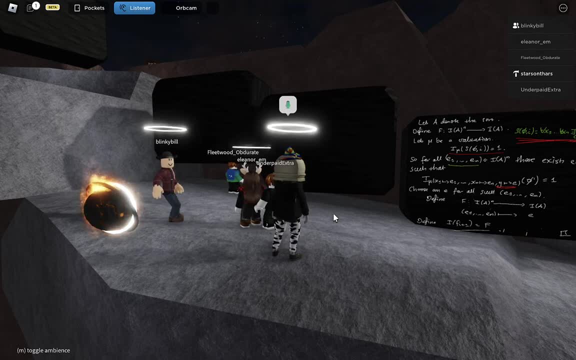 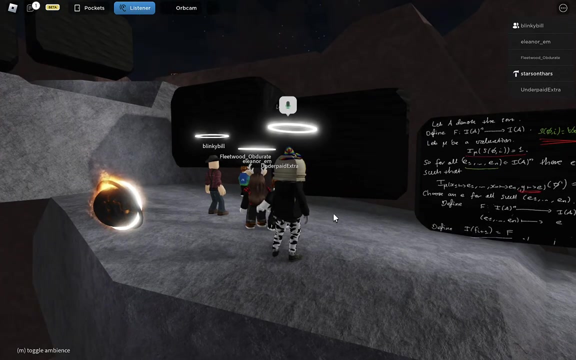 that, uh, if this is all like inside some theory, then fine, you get to use choice in the meta theory, which is just zfc. that's of course fine, but you're going to proceed to talk about it in a way where you aren't thinking about it. exactly like that, i think. yeah, anyway, this is, this is kind of 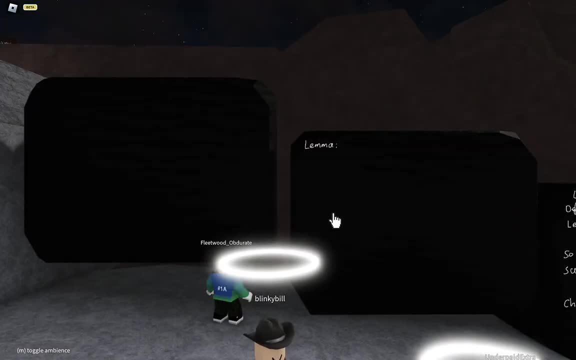 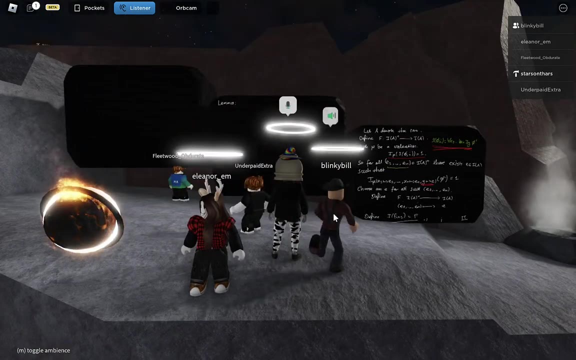 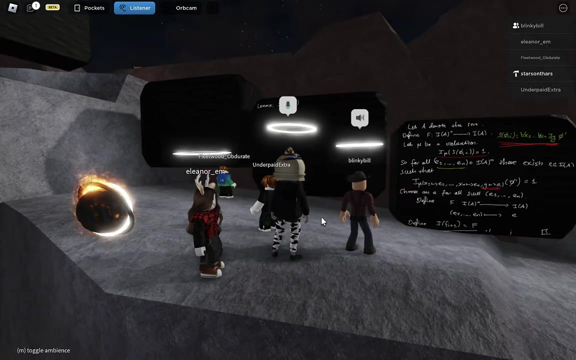 not something we should get derailed on again. i think, sure. um, billy, yeah, your halo is too shiny move. oh, okay, i think, i think you're making too many assumptions where we're going to go with this. okay, i will. i will lurk in my den and wait for you to make a mistake and then i'll rush out. 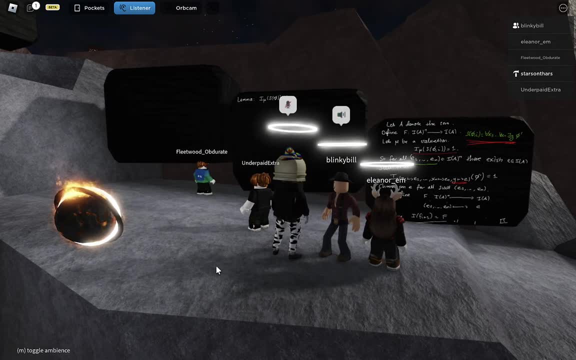 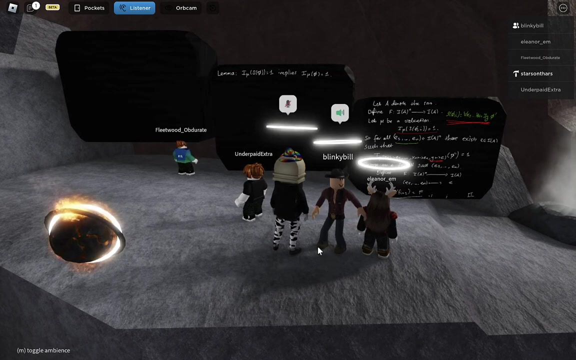 i think this is just normal mathematics and this the things that we do here. you hold to much higher standards of what it's supposed to magically achieve than like regular mathematics that we do in other seminars. my impression so far is we're using a lot of symbols to say something that is kind of obvious. 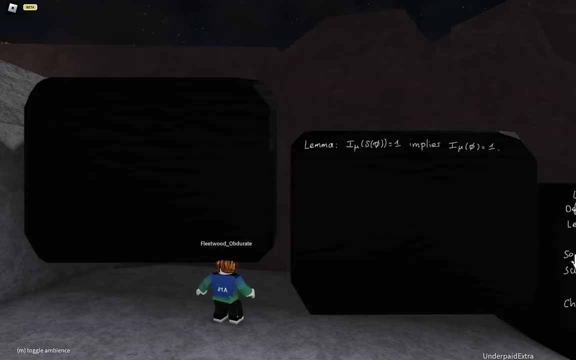 the idea, eleanor, is to pin on what you consider obvious. so we're trying to challenge, like you're. you're saying that picking a representative of these a's for every tuple is obvious. now, that's what you've said there, right, and you can go ahead and hold that opinion, but let's be aware that 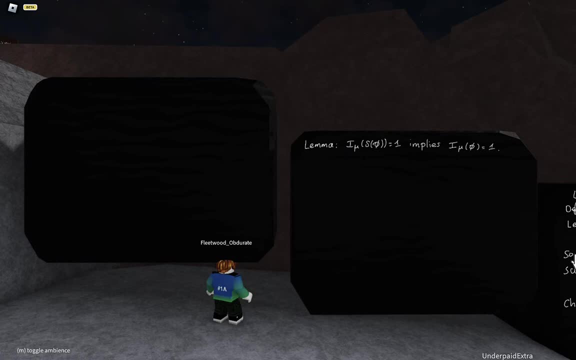 that's what you're saying, and then when you chase that again, it gets pretty weird. um, i was going to. i had a point that i wanted to pin down on, but i forgot. that's actually okay, i'm going to skip the proof of this lemma. it's basically identical to what i just did. it's just in the opposite direction. 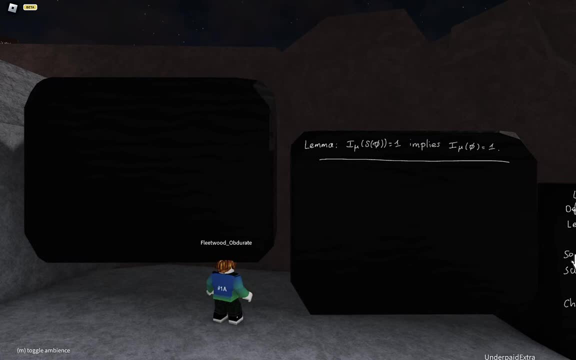 right. so this essentially says that if i have a model for the spilling, then i have a model for the original one. um, but you need to get your, you need to get your assumptions correct. so if i have a- uh, yeah, i know that i have a model for the spilling, so i'm just going to get rid of that one. 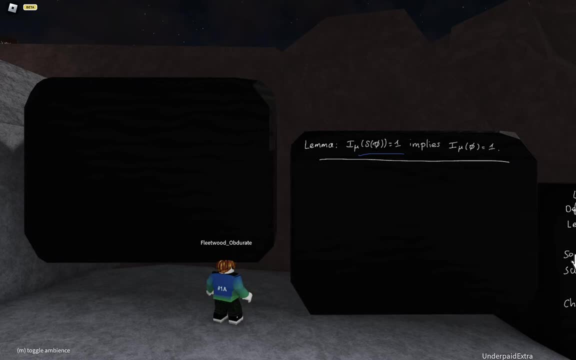 i need to have a model of this colonization that evaluates to one in this particular for this particular choice of formula. so this is for all phi inside some first order theory t, and then i'm just going to lazily write same hypotheses as previous lemma. okay, so it's essentially a converse. 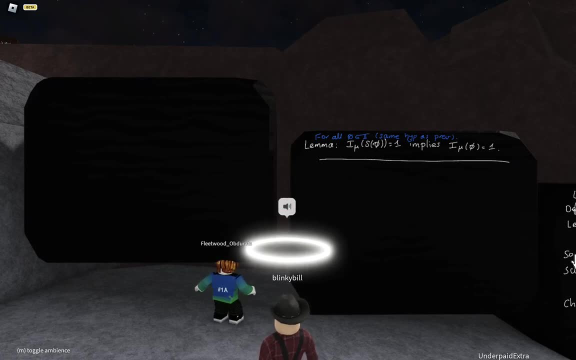 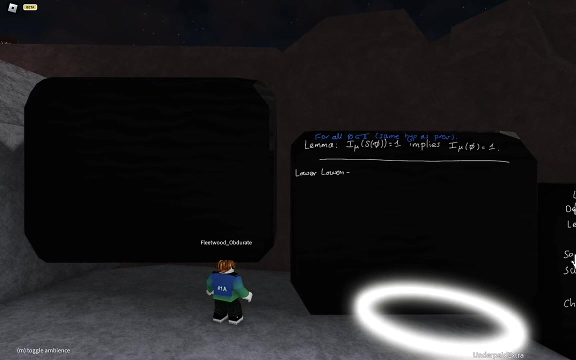 should be like a whole lot less controversial, because we've, yeah, we're starting with all the choices and then we're just removing them and, uh, just reducing them to an existential yeah, yeah, exactly. okay, lower lowenheim's column theorem, the moment we have all been waiting for. 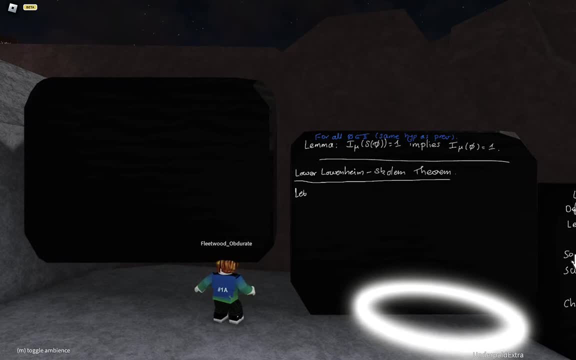 okay, i'm going to write out all of the assumptions that i've been making just to get a very precise statement. t is a first order theory with only one sort and all the formulas are closed and in pre-next normal form. okay, are you ready? are you ready for the hypotheses? so this is going to be a whole. 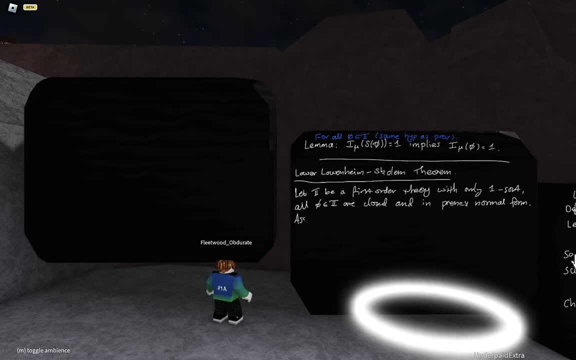 bunch of cardinality stuff. assume, oops, the language t is over has, at most, countably many, many function symbols. Is that it? Yeah, Assume that we have a model. There is a model I of T With the magnitude. So this is the cardinality. 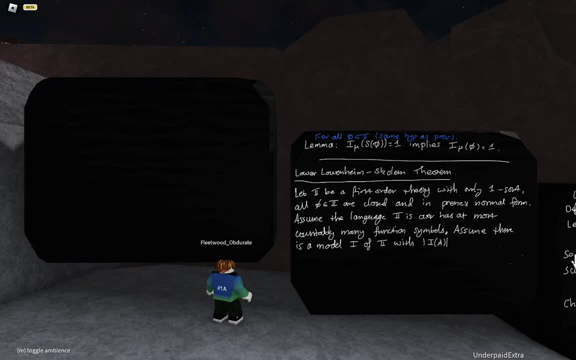 The cardinality of I of A is infinite. So some infinite cardinality, Okay. And then for any cardinal of kappa less than or equal to the magnitude of I of A, So less than or equal to the cardinality of I of A. 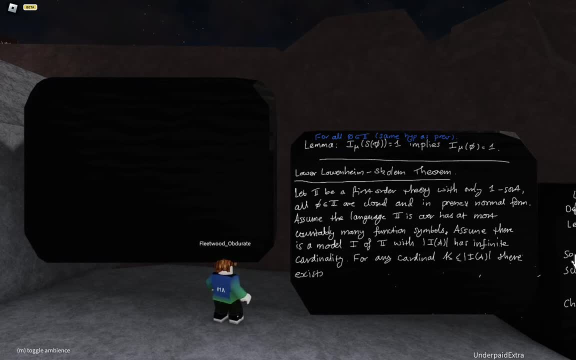 There exists a model J of T with the cardinality of J of A is equal to kappa. Okay, So there's an upper Lowenheim's column theorem as well, which gives us the general Lowenheim's column theorem, But you can see why this is the lower one, right? 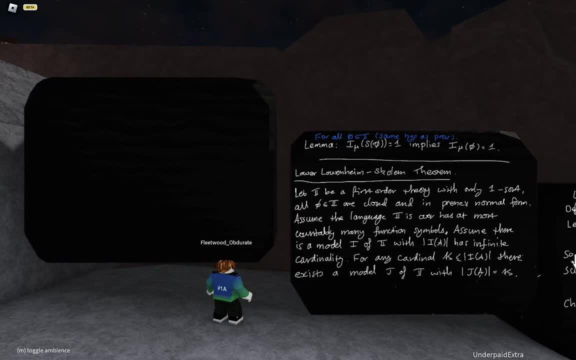 We're just saying that if we have a infinite, if we have an infinite model, then we can get all of the cardinalities less than that model under certain hypotheses. So there are more than one, There are more general statements than this. 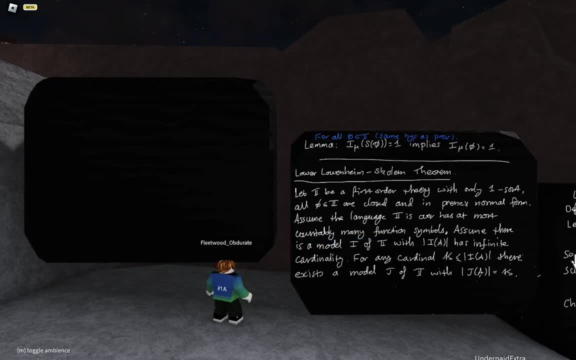 So asking that we have count at most countably many function symbols is just to make the statement and the proof a lot easier. but you can remove that hypothesis and get a weaker statement. It's not necessarily equal to kappa, but it's equal to the maximum of kappa. 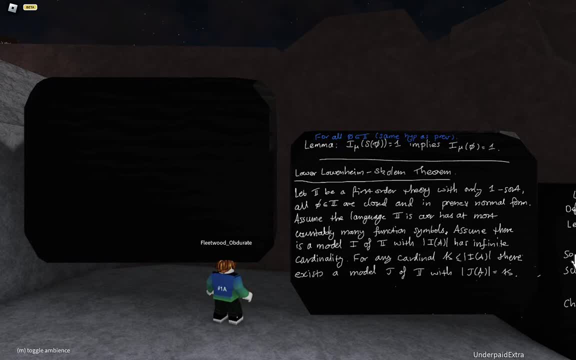 or the cardinality of the set of function symbols that you have, And there's nothing inside this theorem that requires you to only have one sort as well. That's just a simplifying mechanism, because that's all that we need for the Axe-Krofenbeck theorem. 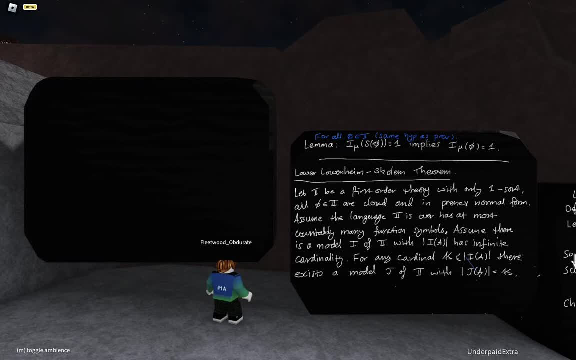 Cool. Is the statement clear? Okay, Yes, Nice Proof, Okay. So let me tell you what we're going to do. It's just a sneaky sleight of hand. I'm going to grab an arbitrary subset of i of a 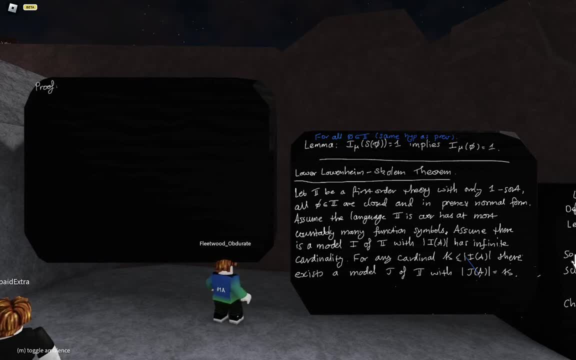 which is of cardinality, kappa, and then I'm going to take the union of that thing along with the image of all of the interpretations of the function symbols of the language, Now, since I've only got countable at most, countably infinitely. 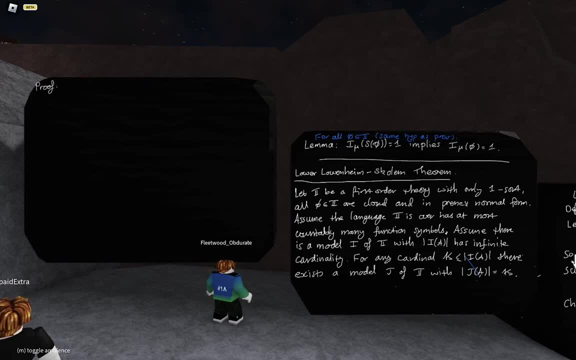 many function symbols. the union of the subset of cardinality, kappa, and all of those images is kappa, right, But if I think about that model, it has the images of all of the function symbols inside it, and so I can definitely create a model inside that. 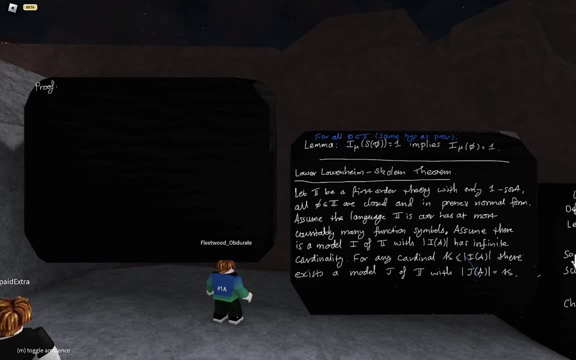 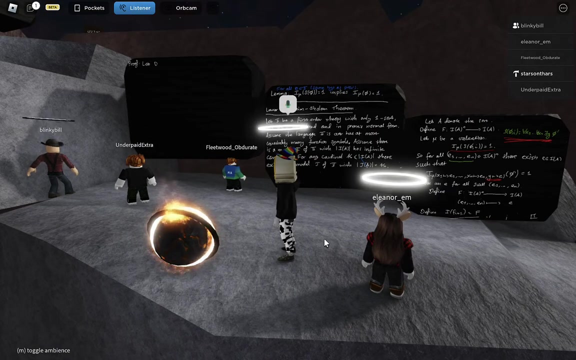 I'm basically just restricting the model down to the minimum that I need, which are the images of the function symbols, and then, like, extend it arbitrarily out to some set of size kappa, and then we're done. okay, Did I not say that? 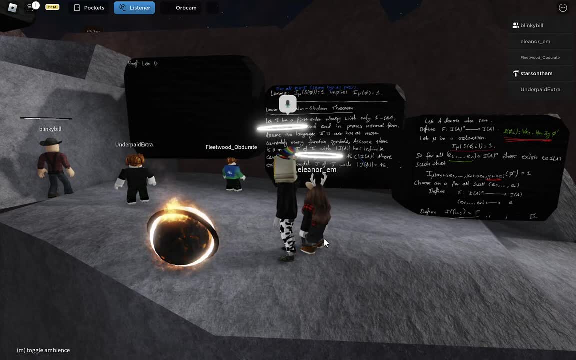 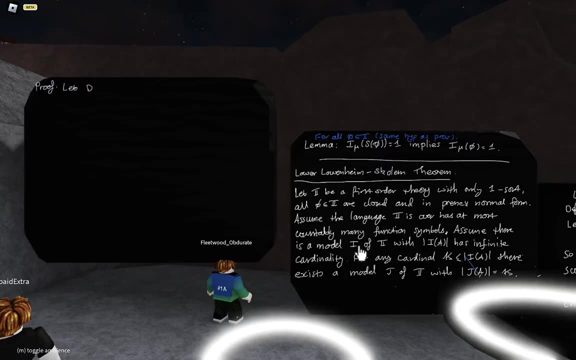 No, you didn't. I was also wondering this, So in the statement did I not say it. Let me have a look. You didn't yeah, Ah, okay, yeah, that's important. Oh, for any cardinal. yeah, that's not right. 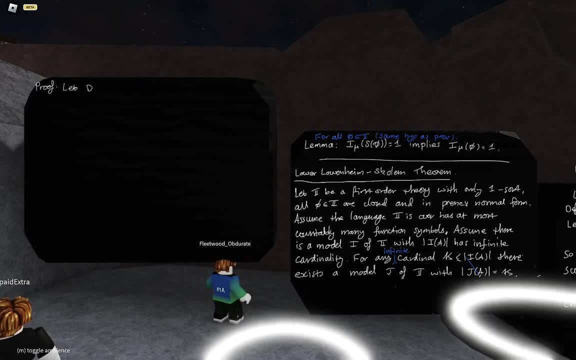 For any infinite cardinal. Okay, good, pick up, thanks. Let D subset of R of A be an arbitrary subset of cardinality. kappa, okay, And now. yeah, I'm going to consider a scolomization of the first-order theory. 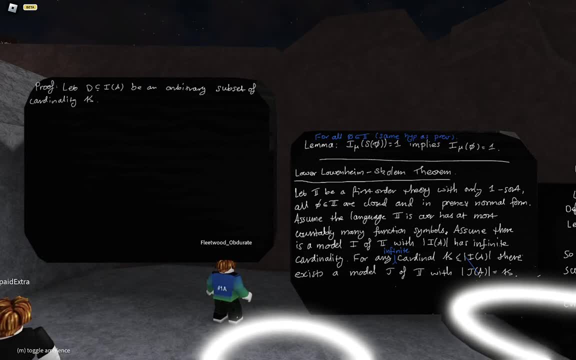 And the reason why is because the interpretation might end up picking an element of I, of A, which lies outside the images of the interpretations of the function symbols of T, when I have to interpret an existential quantifier. So if I remove all of the existential quantifiers first, 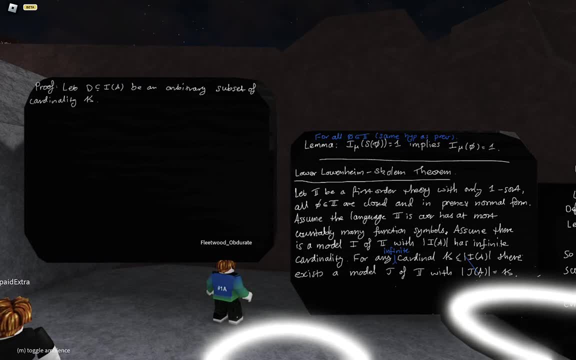 then I can control the codomain. So if I remove all of the existential quantifiers first, then I can control the codomain. I can control the codomain using the function symbols. That's the whole reason why we need a scolomization. 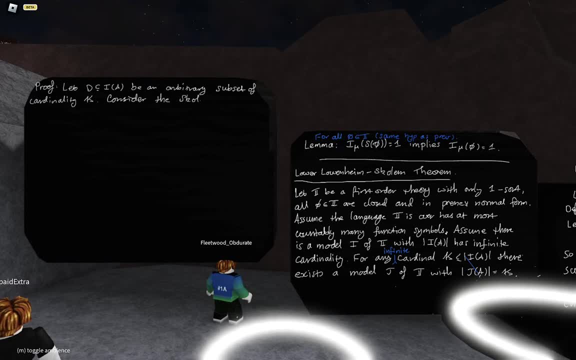 by the way. so that's the crucial point in the proof where scolomization is used. Okay, That was enough, everybody. I'm trying just to copyright the co SOLENE. Okay, Thanks guys. See you next time Okay. 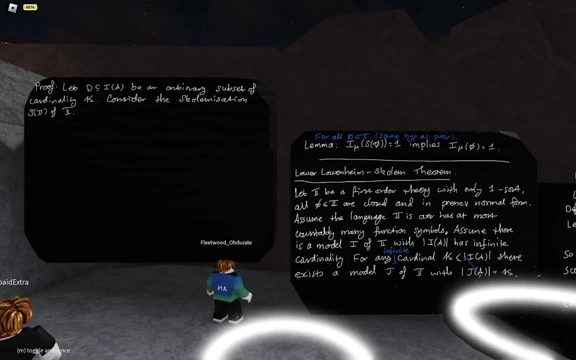 And then we've already proven, we proved earlier- that since we have a model of T, we have a model of the spelumization of T. Cool, Okay, now let's look at all of the function symbols inside the spelumization of T. 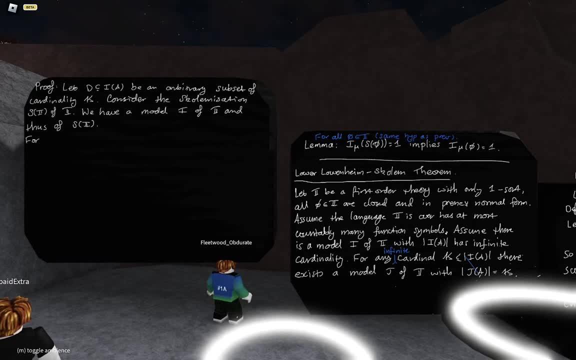 This is going to include all of the spelum functions, So to each of these I consider the image of the interpretation. So I take image of the interpretation of F. sorry, restrict it down to D. right, Because I can just go ahead and restrict the domain of the valuations to D. 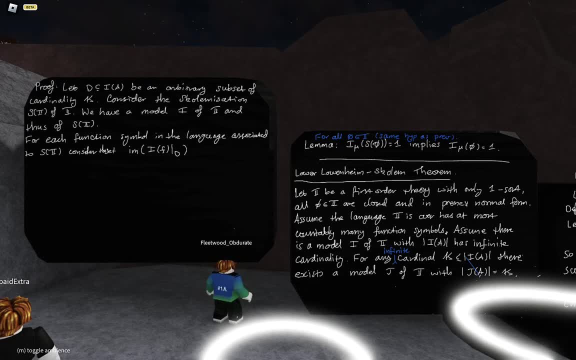 And then I do the same for my function symbols, and we still end up with an interpretation. Okay, so pick an arbitrary valuation, nu. And now the set that I define- and this is going to be the domain of my PAPA- in cardinality model is E, which is the set D. 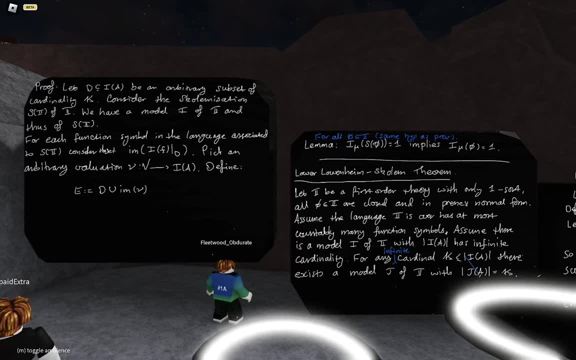 And then I union the image of nu and I union the big union of all taking, you know, over all of the function symbols of the image of I, of F restricted to D. okay, Now, this is the most important step in the proof, this definition, along with the observation that it works. 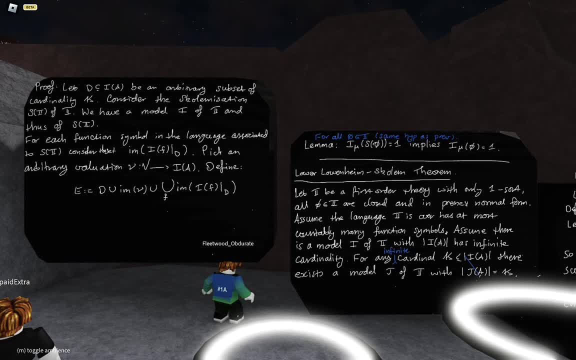 So the first thing that you need to make sure of is that you have indeed ended up with something that is well-defined. Taking all of these Images is what is needed, because we're taking functions out of the set D, because they're all restricted down to D. 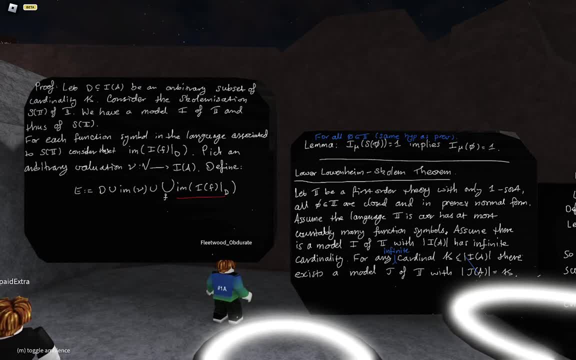 But I need to make sure that I end up with elements inside my domain, And so I just union all of the images to guarantee that. okay, And then we need to make sure that this has the correct cardinality, And the observation is that this has cardinality. 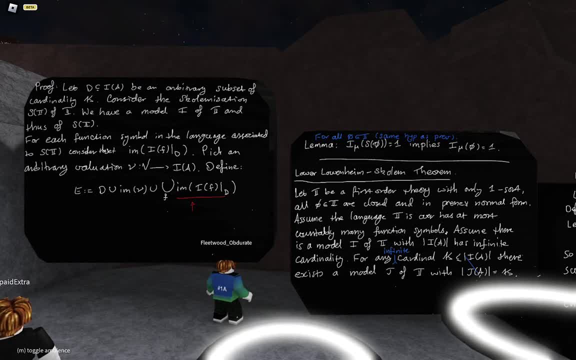 This should have both of these values, This should have all of the values, And then we need to take that one for reference in the order to make sure that it's more or less than or equal to our left null right, Because there were, at most countably, infinitely many function symbols. 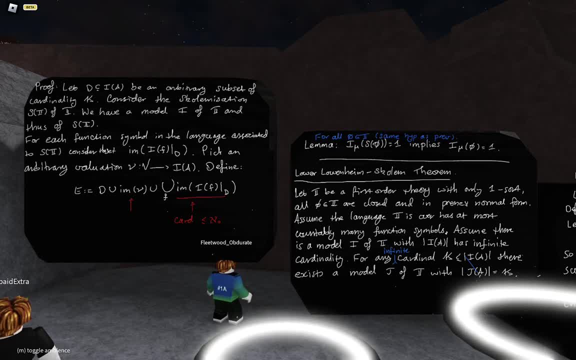 The image of the valuation. well, if you go all the way back to when we defined first order theories and first order languages, we said that there is a countably infinite set of variables. the image of this set is: has cardinality, also, less than or equal to LF, null. okay, and then d. 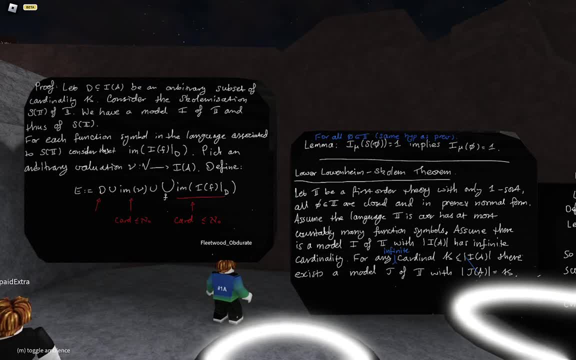 is the arbitrary subset of cardinality kappa that we took right at the very start. so this has cardinality equal to kappa. okay, kappa is at least infinite. so therefore the cardinality of e is equal to kappa. does that make sense? so, as I said, that's the most important part of the proof. 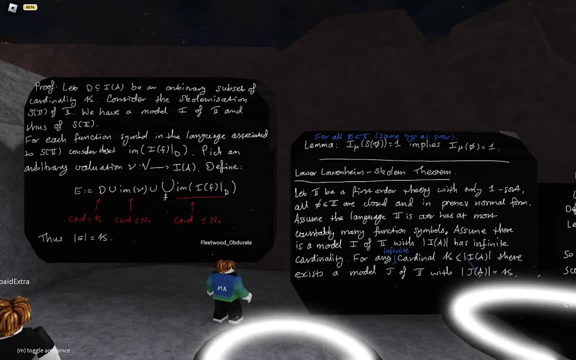 and then the rest is just to check that this indeed works. so let's, let's go up a layer. wait, I actually had a question. yep, if we started with only finally many function symbols and variables, like, of course, that's a like, you don't want to have finally many variables, but just 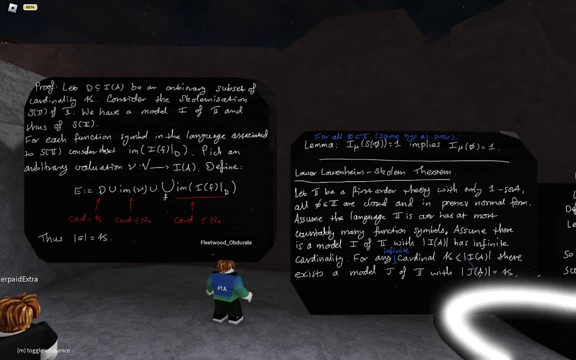 because of this theorem, could we drop the infinite cardinal assumption on kappa question, like that would make all this still work, right? I think that kappa would have to be a cardinal greater than or equal to the maximum of the cardinality of your variable set or the cardinality of your function symbol set, and then I think it works right. yeah, yeah, you need. 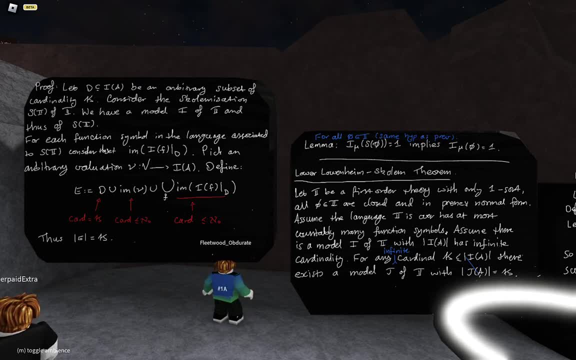 the cardinality of d to be- oh wait, there might be more to it than that, because the cardinality of this union is now going to be additive, right? so yeah, yeah, I think, sorry, yeah, okay, yeah, um, and if you did that, by the way, that that would be insufficient for the. 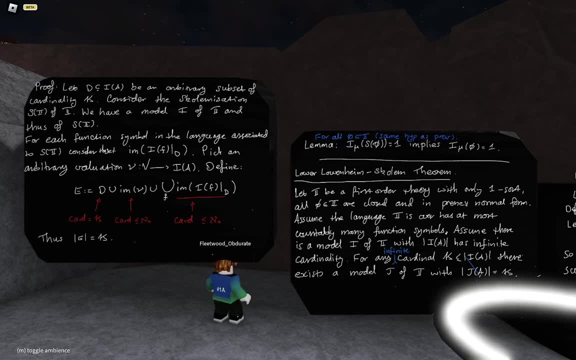 Axe-Groven-Dick theorem. okay, because the first order theory of algebraically closed fields of characteristic zero had infinitely many um formulas and so you've got infinitely many, uh, scolom functions. so you have infinitely many function symbols, right, right, right um. the other one was: so the lower moment scolom theorem is clearly. 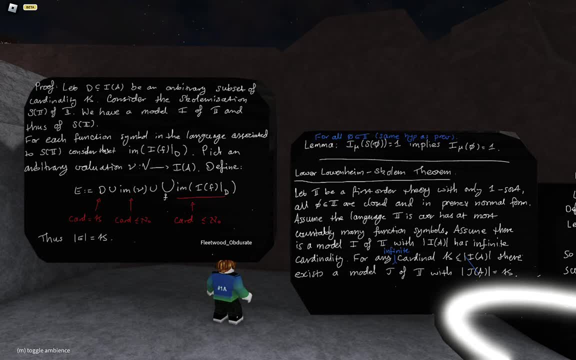 like clearly about the existential quantifiers and things like this to me, how do you use this compensation? um, yeah, there's. yeah, there's a set of existential quantifiers, the set of objects that are getting bigger and bigger, but for all of them, like universal quantifiers, like we don't really care, they're making the set of things smaller. so 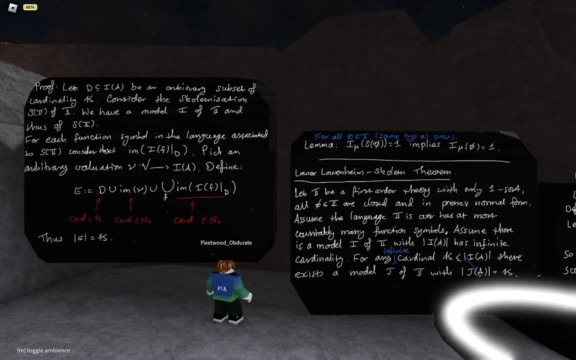 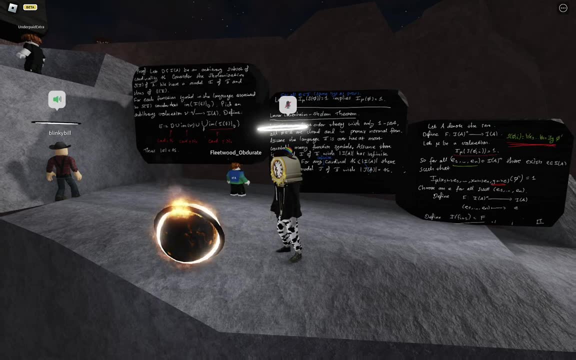 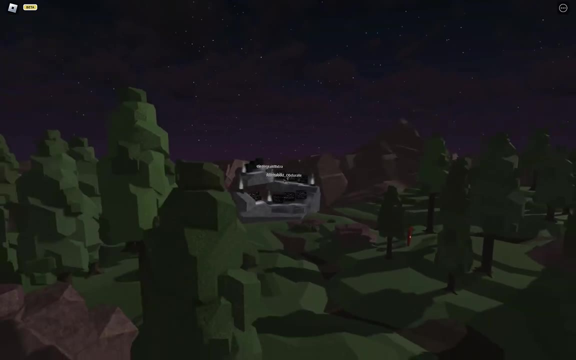 like a universal exactly quantified like remain true? um in the in the upper lowenheim scolom theorem. do you have to like concern yourself with the universal quantifiers in a dual way or yes, that's a? that's a really good question. you don't, because 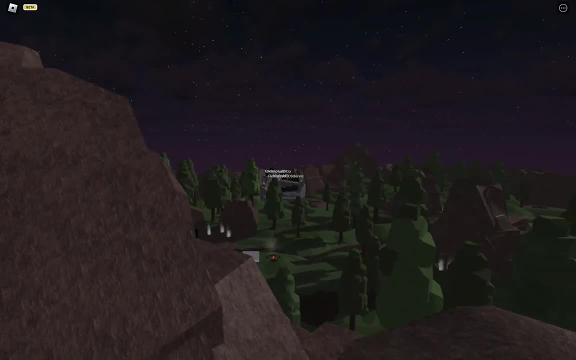 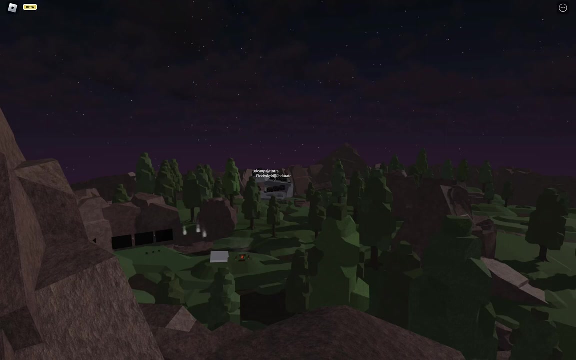 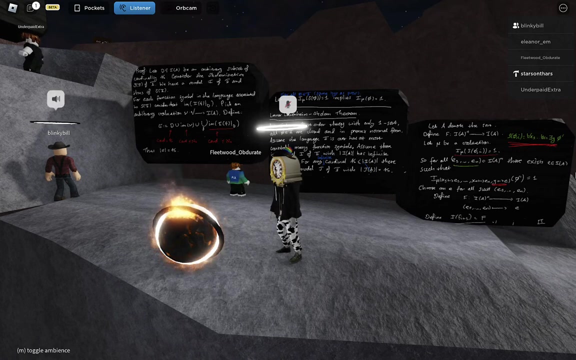 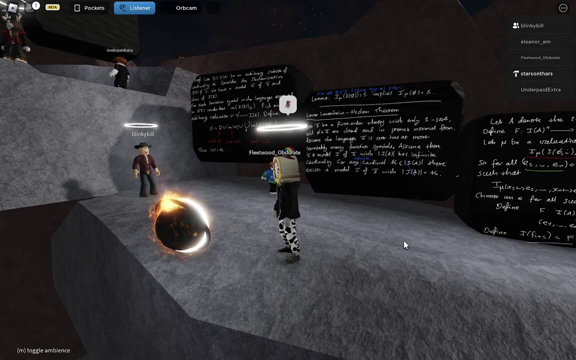 there's a slip trick that happens when you get to the upper um, like upper lowenheim skull theorem. oh, I like your, i like your thinking um. look, probably both techniques will work right. but what we're going to do is just introduce a set of cardinality kappa worth of constants, right, and then they just add all of. these formulas to the theory. let's say the uh example, for example, of this thing is a threshold for this machine, perhaps because it's called cardinality kappa. it means that that'll be fair to insert, which is: if momentarily aesperius times kappa minus x equals الك in constant time. but that means that in the past it was possible. toриun, smiling, was said that this is a 가ussal toward you. it's possible that when you seeds on the Trumpdam, as we 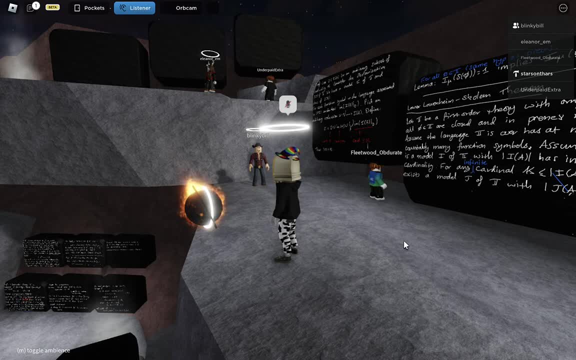 the theory that say these, every pair of these constants are not equal to each other. and then, yeah see, it's like simple g. and then, and then what i do is i use the fact that we have the compactness theorem. so, since i have, um, all finite models of that, because i can always 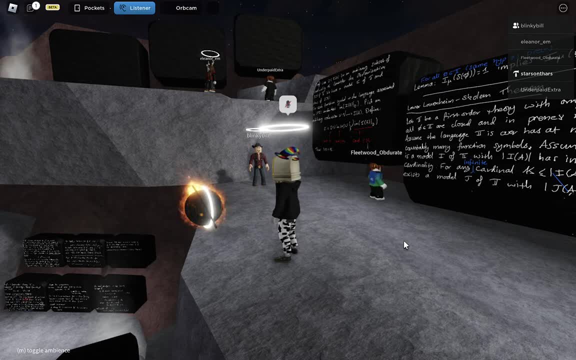 just pick uh for any n n elements of my infinite cardinality model and get distinct elements and all of the formulas are provable and hold inside that model. i can do that for all finite subsets and so therefore i get some infinite cardinality which is at least greater than or equal to. 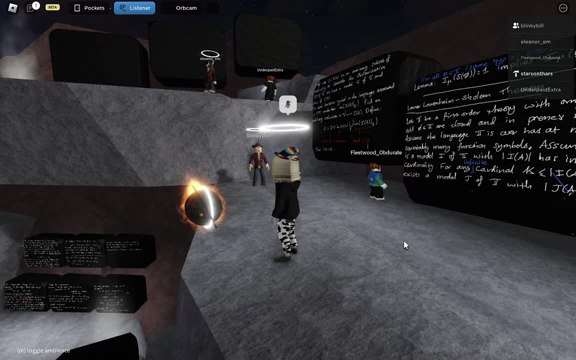 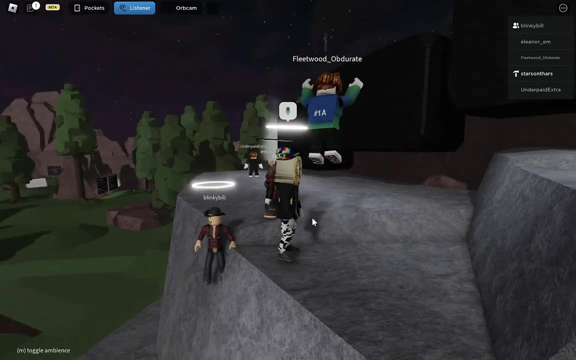 kappa, because we have to accommodate for all of the constants. and then i appeal to the lower loewenheim's column theorem to shrink the possibly too big thing back down to exactly kappa. all right, right, so that's the trick that will be used. tell me again how logic is a dignified discipline. 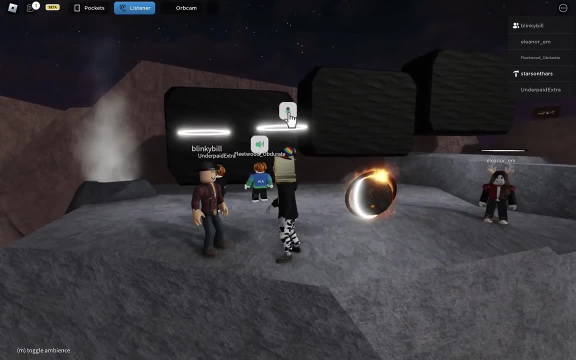 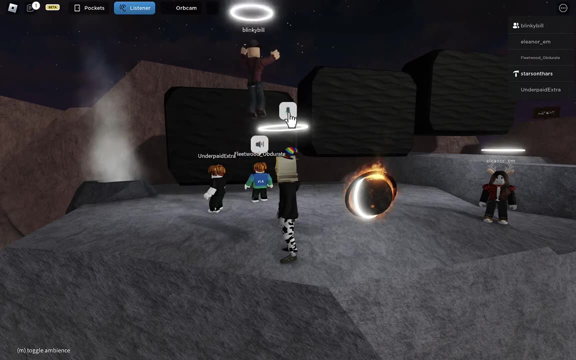 no offense, dan, if you want to be invited to future lectures. yeah, no offense. okay, i can learn to be a little bit more polite of the world. look like i. i don't want to. i don't encourage your rudeness, but i see you know your point. um, i find it surprising that all of this is needed for acts as well, is the thing so? 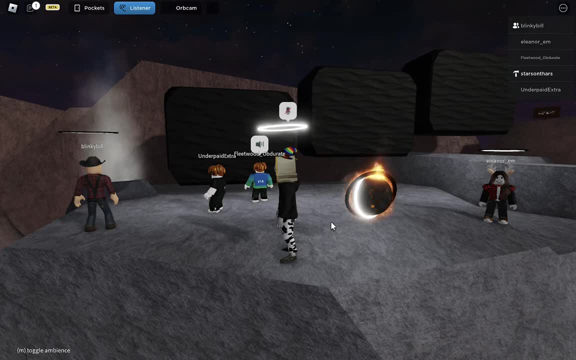 this is where i really got the bullet, that this surely wasn't how they proved it originally. at least this content wasn't invented by the axe growth. indeed, that that much certainly is true. but i wonder if you can just specialize everything and get down to a much simpler argument. but yeah, 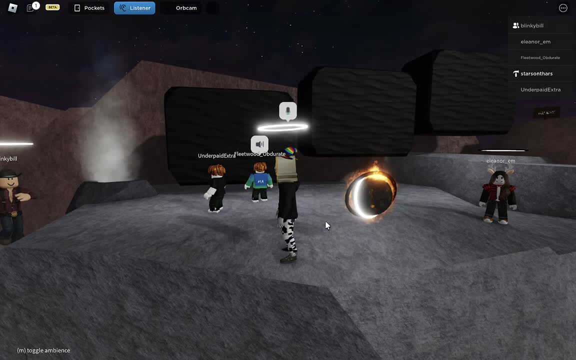 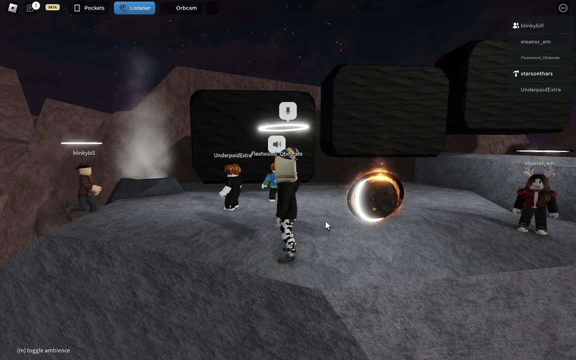 there's a lot of ad hoc stuff inside first order logic and it's part of my complaint, or first order logic i i would expect the world's most natural logical system to not have so many ad hoc movements, like even the pre-next normal form like come on, really, i can't believe that i have. 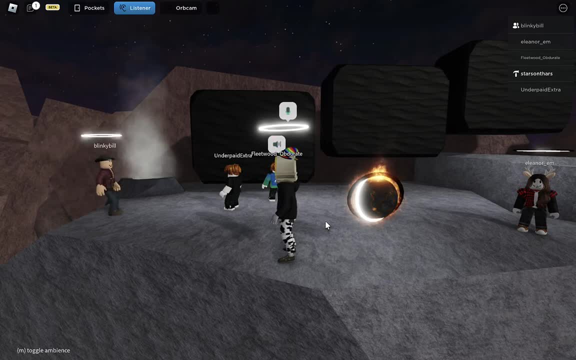 to do all of that, and these are questions to be explored. i guess i'm willing to believe there are- that this ad hoc stuff is is not really significant and i'm just not seeing the ideas clearly. and that's no criticism of you, but a a it does. i'm just communicating the feeling i have listening to this is it's kind of like yeah, okay. 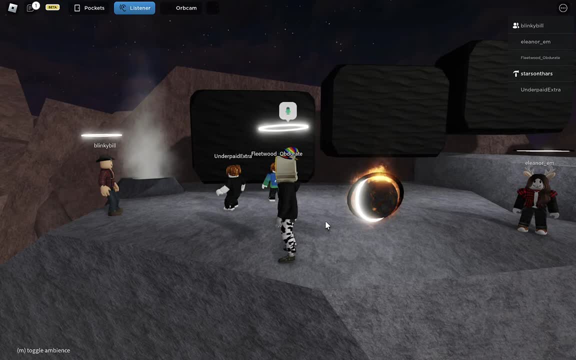 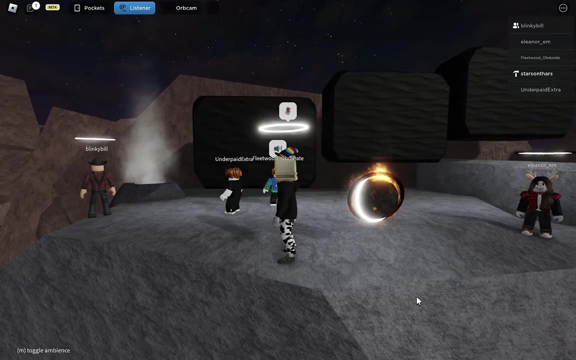 uh, it doesn't, i'm not. i'm not seeing the deep thing happening in front of me, which is okay, uh, but yeah, yeah, i, i have a lot of the same feeling. so the common slogan for the loewenheim spell and theorem is that first order logic can't internally tell the difference between the ad hoc and the 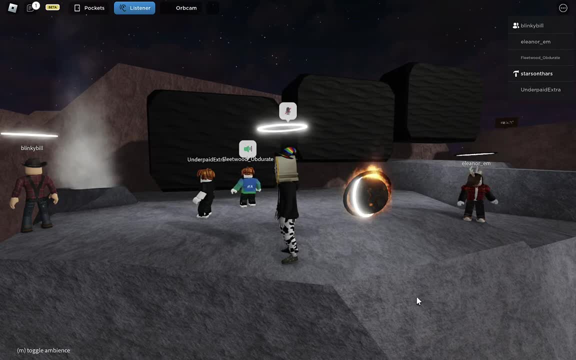 second order logic can't internally tell the difference between cardinalities, right? so maybe that's what the short coming of it is. it's like you have some finite system and so you can indirectly talk about, uh, higher cardinalities, and maybe you could interact with computably. 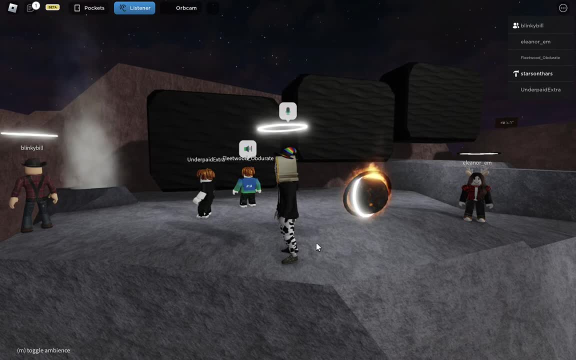 countably infinite sense. okay, we as humans can never. yeah, that sentence you just said made. okay. now, this childish looking operation you just described, uh, has a clear conceptual content for me. so i, i withdraw my, my tantrum, throwing um your head. your head is in the way. 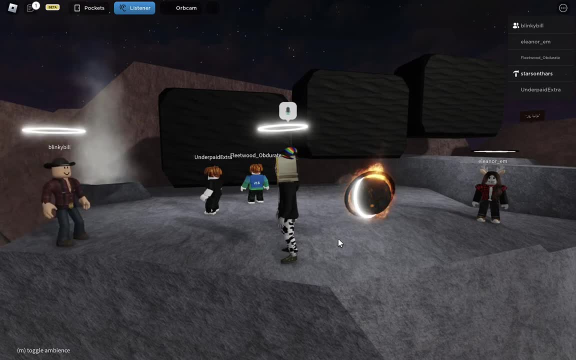 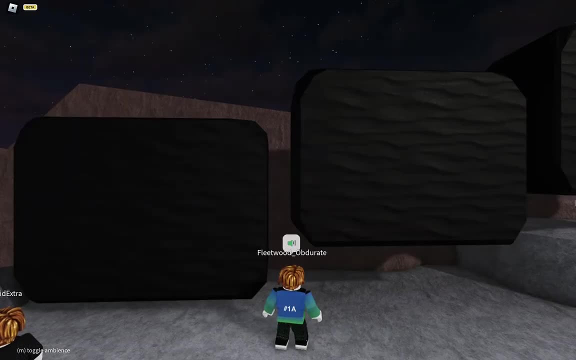 of the board, though before you start writing on it in the orb, cam my head. yeah, okay, all right, thanks, uh, okay, i really want to finish this proof, so so i mean, we're basically done right. so we define the model j. j of a is going to be a set, e, which i'm just defined, and then for all the function, 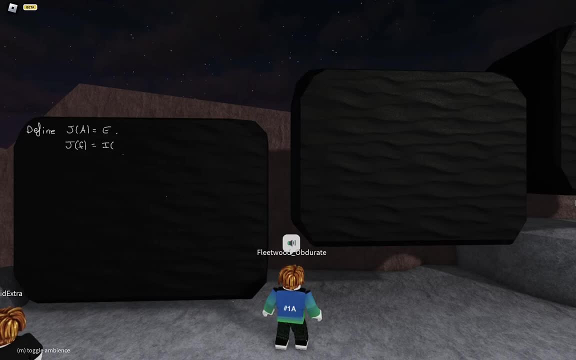 symbols. i define j of f to be the function that i interpreted f with using i, but i just restrict it down to d uh d, to the l right, where l is the arity of f, and then the relation symbols. they don't map back into. uh e, keep in mind that relation symbols are interpreted as predicates they map into either. 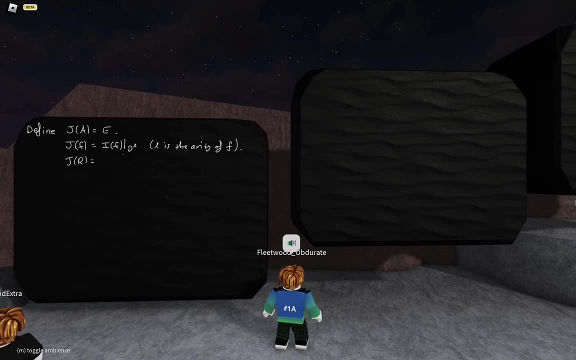 zero or one. so i don't need to do anything to the relation symbols except restrict their domain. cool, and now? now when we're done, right. so the observation is that everything uh gets interpreted in exactly the same way. i've just cut away, uh, a whole portion of the set i of a, which is not visible to any particular element of this. 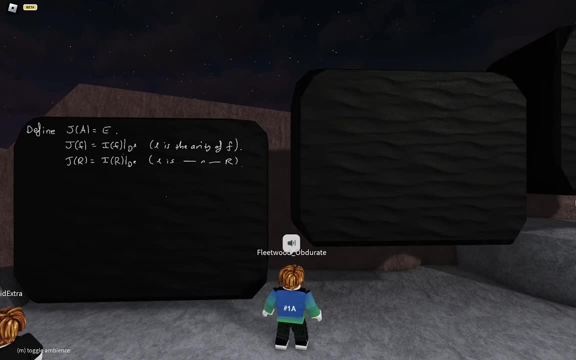 interpretation. so no domain of any interpretation of the function symbols, no codomain, no domain of the relation symbols. ever see those extra elements here. so at the high end of this interpretation. so for elements. So if I want to just do the interpretations, everything's interpreted. 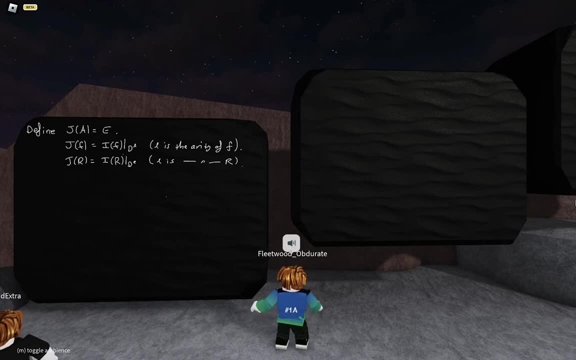 exactly in the same way And so obviously j of phi. so the observation is that j of s of phi is equal to i of s of phi is equal to 1 for all phi in t, And then by the lemma that I didn't prove. 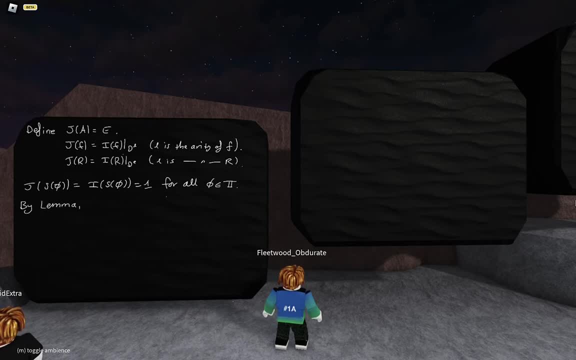 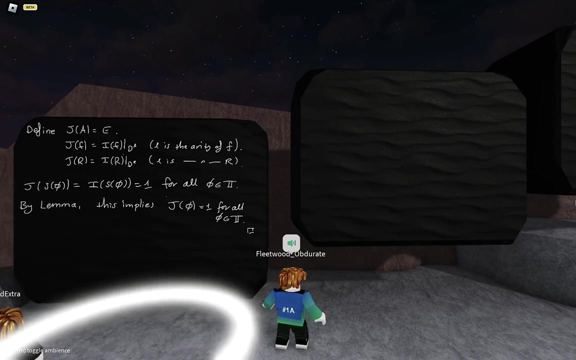 this implies j of phi is equal to 1 for all phi in elements of t. I used both directions inside this proof. I used the first one a few boards back, and then this one. I just used the one that I didn't prove Make sense. 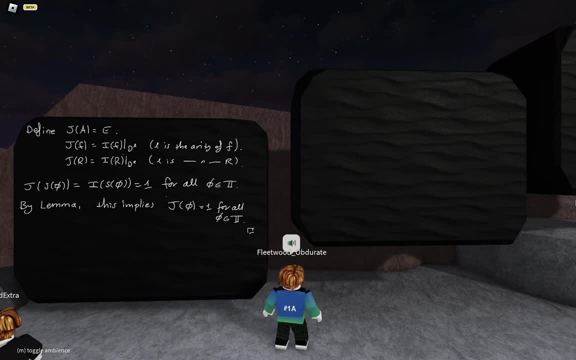 Yeah, Okay, good, Okay, cool. So that's the Lohenheim Spolum theorem. I'm concluding now. There is also an upper Lohenheim Spolum. That's going to be next time, And just to let you all feel like the line at the end of the time. 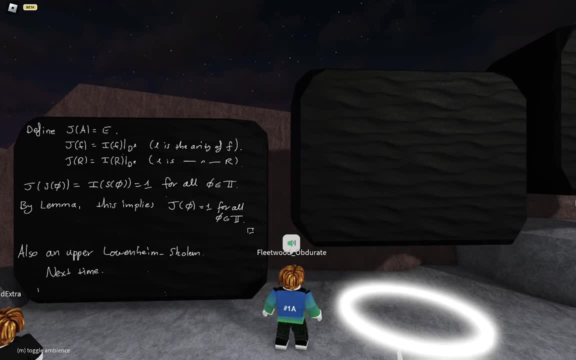 is starting to appear. This is all going to imply the- I can't pronounce this guy's name- the Vosch, Vosch, Vosch, Vosch, Vosch, Vosch, Vosch test. 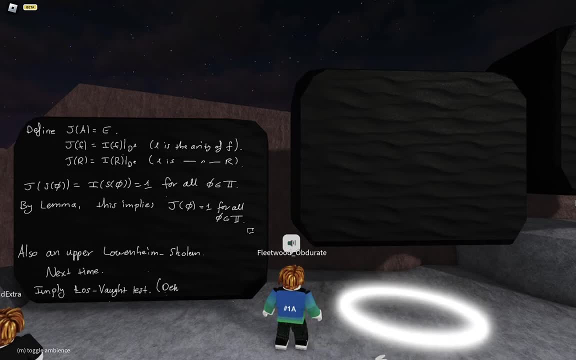 which determines completeness of a theory. Okay, And then I just make the observation that the first order theories of algebraically closed fields of characteristic p and also algebraically closed fields of zero characteristic satisfy the hypotheses of the Vosch-Vosch test, And so therefore, those are complete theories. 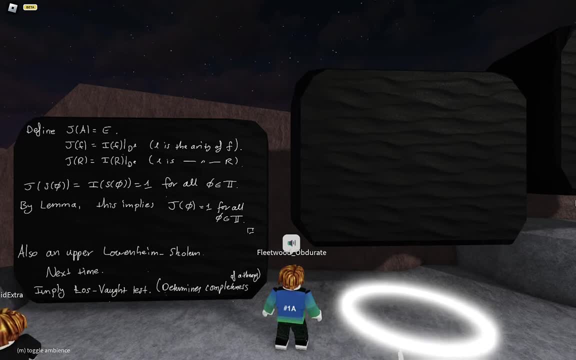 And that was all that I needed to finish the proof. We've already completed the proof of Axe-Grofen-Dijk under that hypothesis And so once we have this, we have that hypothesis And then we're done. So I shouldn't be able to finish next time. 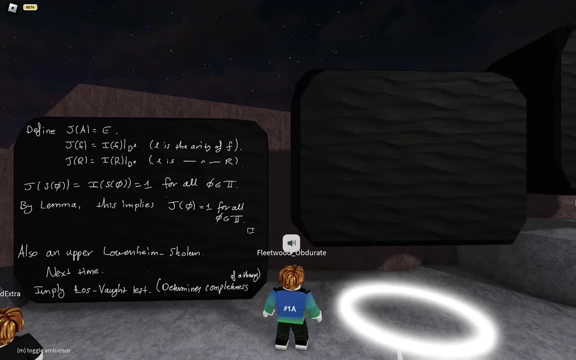 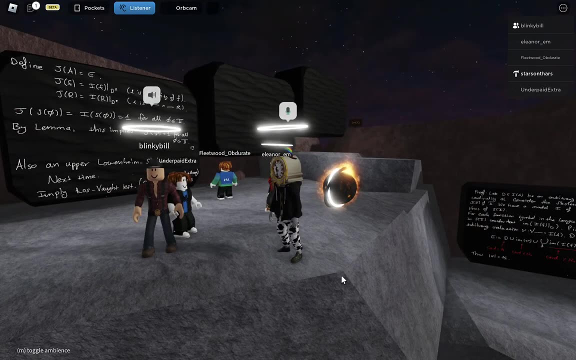 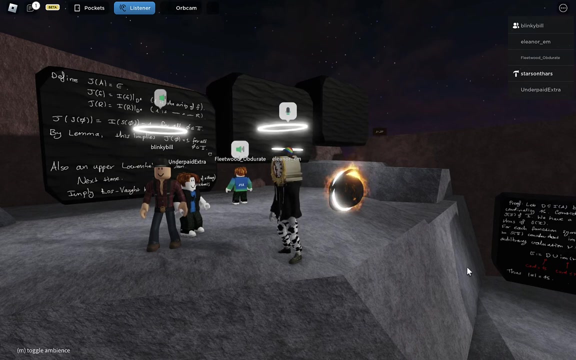 Okay, Thanks and best of luck. Hey, thanks guys. You're welcome. What you were saying about the upper Lohenheim-Spolum theorem, about how like start with your theory- or I guess this applies to the lower one, where you sort of change the theory and then you get this. 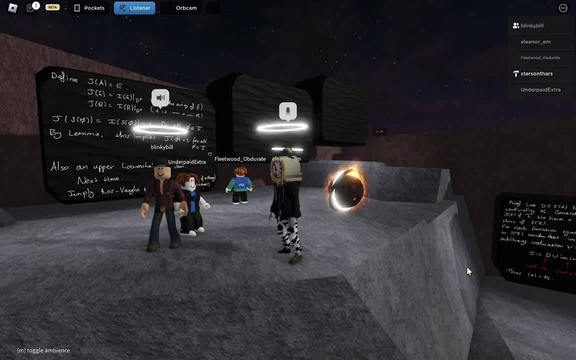 you get this other theory, that kind of or this other model that kind of ruins your day because you're trying very hard with first-order logic to sort of pin down a cardinality. It sort of reminded me of like- I don't know, like a little bit of like the halting problem. 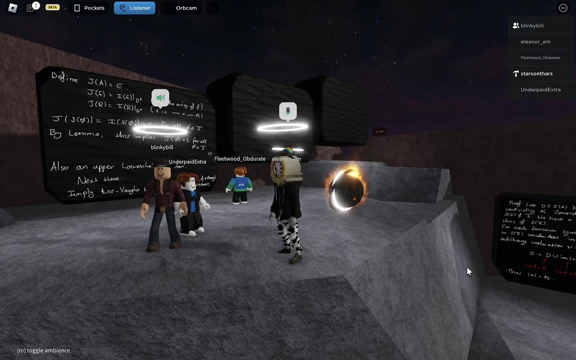 for Turing machine, Like when you're trying to in a particular domain, like you have a, you have a problem that's equivalent to solving the halting problem, but you think you can solve it by, like, trying to detect all these little cases and then that like. 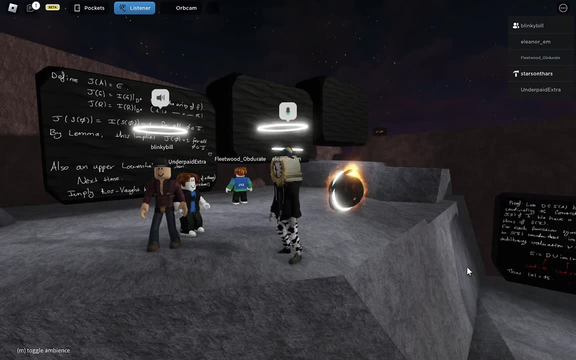 there's just like there's always just one like sneaky case that sort of evades everything that you've attempted so far. Yeah, it kind of reminded me of this. I guess I had both these feelings with the first-and-completeness theorem, then here, 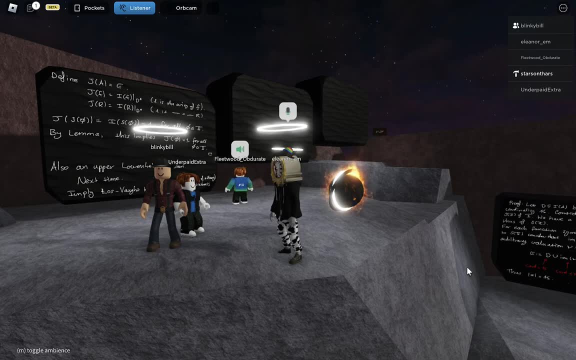 I had both these feelings with the first-and-completeness theorem. then here, I had both these feelings with the first-and-completeness theorem. then here, Mm, Because that's the point, Because that's the point, My reaction to like the like when I first saw the proof of the that 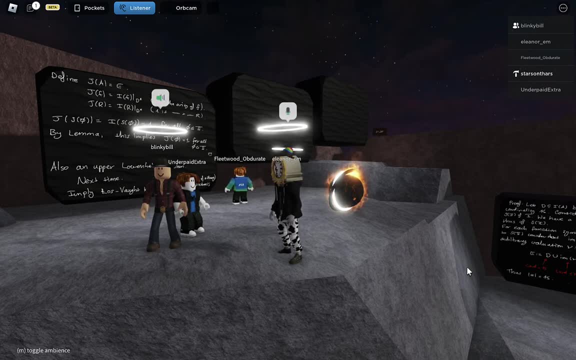 that, like there's no Turing machine that decides whether a Turing machine will halt. It's like, oh, why can't you just? well, I really care that. like it doesn't work when you run it on itself, Mm. 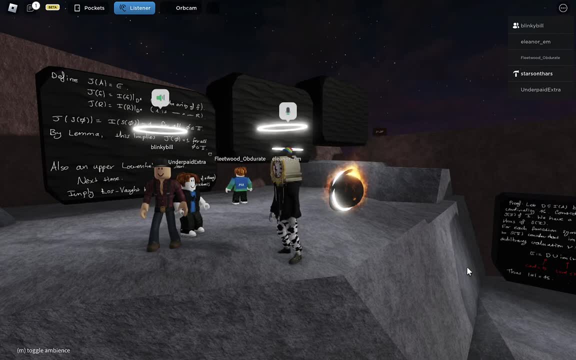 self, or something like: what if i could just decide if all the normal sensible turing machines hold and not just this, this like um pathological counterexample: turing machine that like, ruins the, the fullness of its ability to, to detect, holding um so, so like in that way i like, i guess. 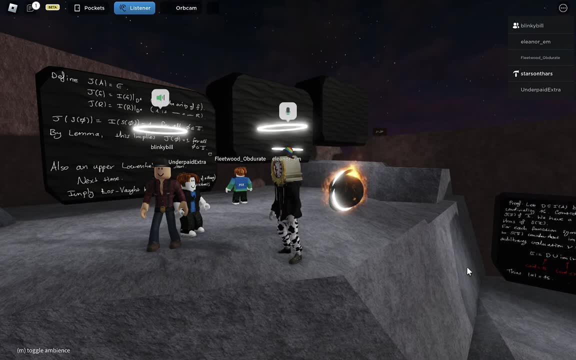 i'm. i'm sort of addressing the idea that like these modifications of the theory, like like this one where you chuck in all these extra constants and say they're all not equal, like we obviously do not care about that particular theory for any practical purposes. but it's like 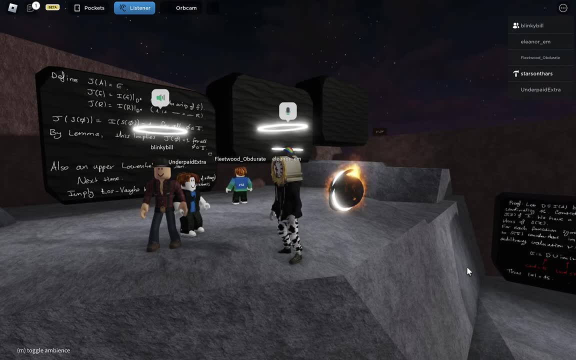 but it's just the sort of pathological thing that can happen within the realm of what, um, what we say can count in first-order logic as a theory. that, um, that sort of, is the reason why first-order logic can't distinguish cardinalities. very well, interesting. so the way that i think about that trick that we're going to use, 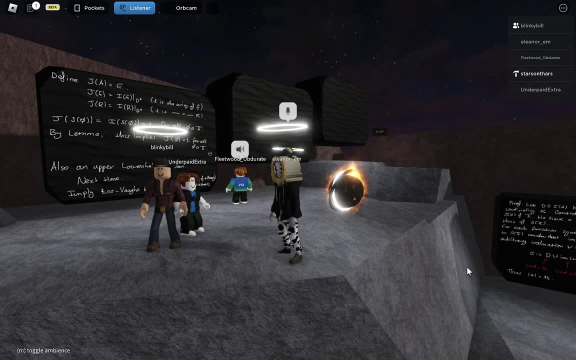 is that there is a clear relationship between the original model and that one in terms of in this kind of this inject injection, like if you take your first order theory and you just add a bunch of constants that you don't really care about and then you extend your model to care about those constants but that extra model is basically. 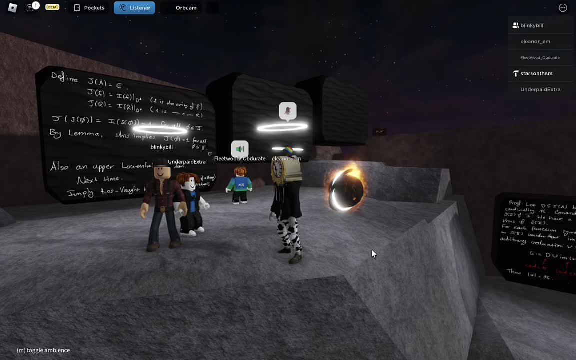 a disjoint union. there's the original model disjoint union, another set out there that just handles these extra constants, right, then the point is: uh, there's no barrier to injecting some lower cardinality model into a higher one, right? so if i can prove something to be true inside some lower cardinal model, then i can just increase that set and i don't. 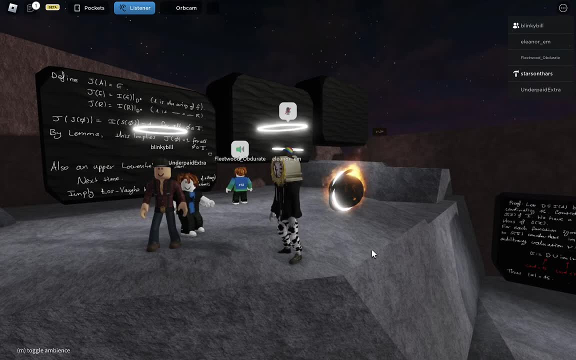 now lose truthhood of that of that statement, right? so it's like non-pathological almost, because that would be weird if i could add stuff that we don't care about and all of a sudden the statement becomes false, right, anyway. and the reason why that's um. 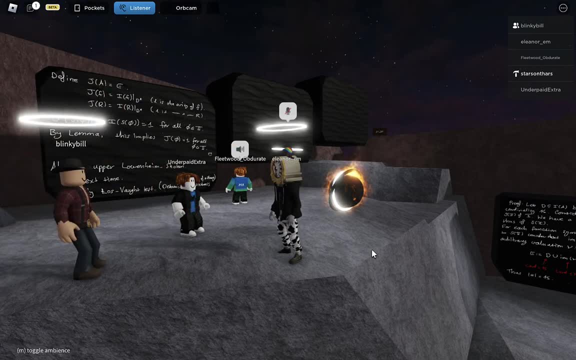 interesting is because if i can prove something to be true inside some lower cardinal model. interesting is because if i have a statement that is prove provable and also its negation is provable inside the same cardinality model, then i can do a bijection argument and carry truth. 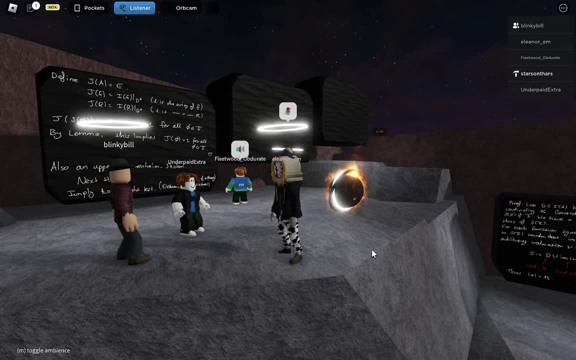 through, um, that bijection which is going to give us a contradiction, which is going to prove the uh, the wash for test. so the point is that all i'm really saying is i've got these two models, one's bigger than the other- who cares? like one's an extension of the other right, and the formula is true in one of them, and 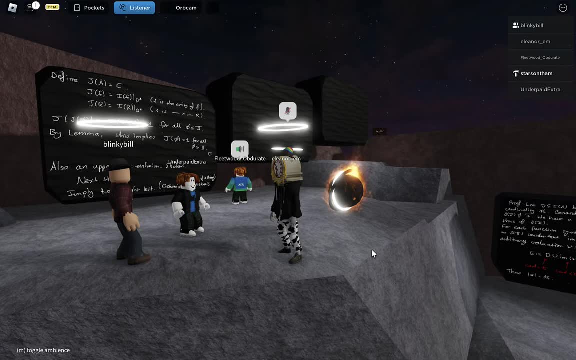 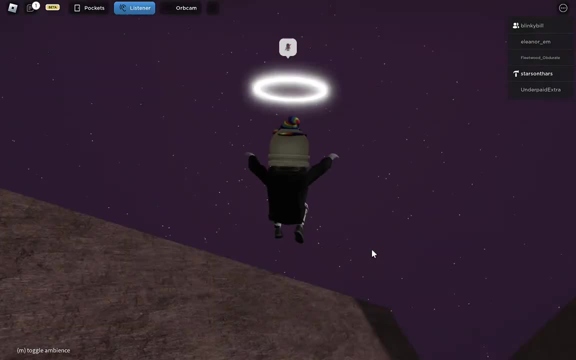 it's false in the other one, and the point is that is a contradiction. you might say, oh, how do you know like those models are of different cardinalities? you need to set up some map from one into the other and check. it's like you kind of roll your eyes and you're like, yeah, sure, fine, but then you 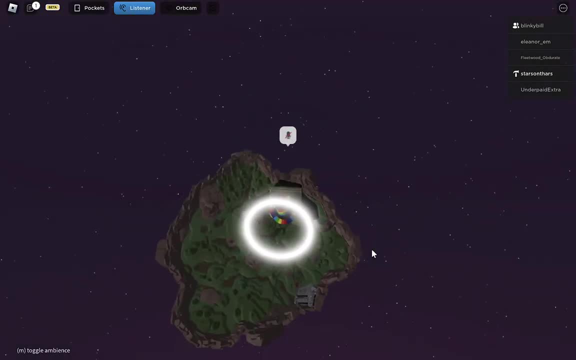 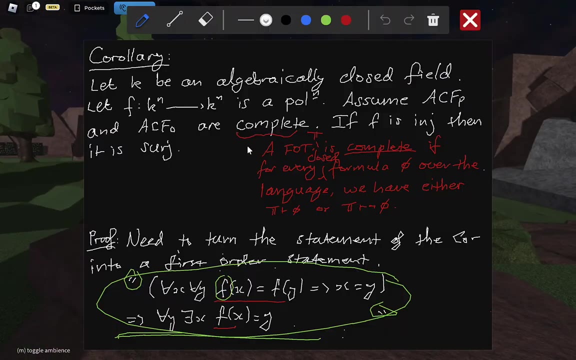 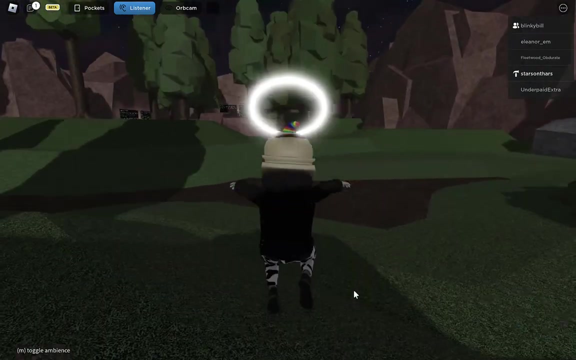 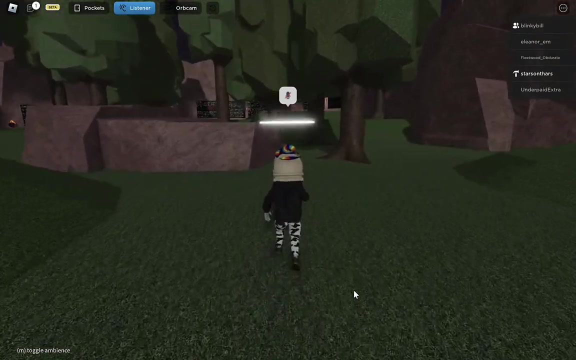 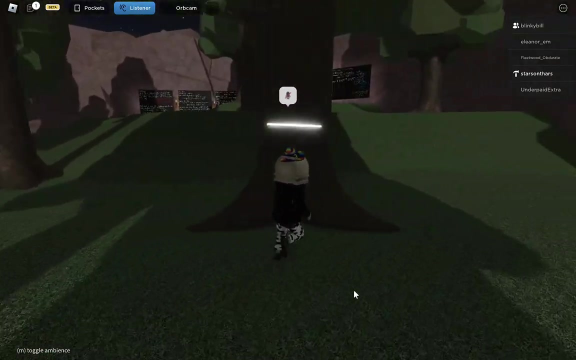 do that and it does work. so i think it's more about relating extensions and restrictions of models, and we use the language of cardinality to describe it, because we use bijections in order to carry truth between models. that's really what's happening, yeah, so there is tons of redundancy. i would be very interested in some modification to first. 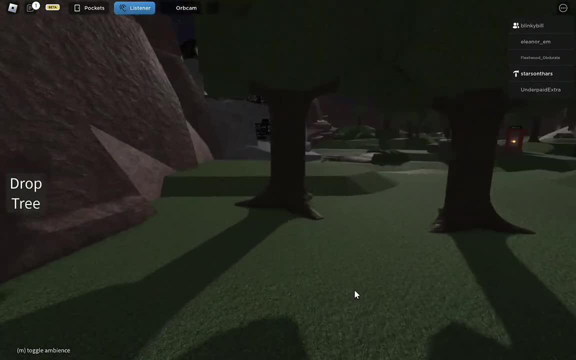 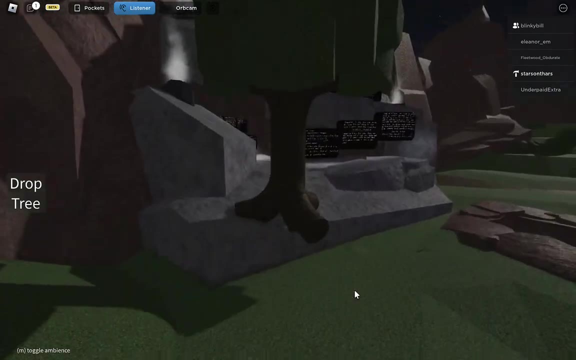 order logic where these redundancies don't have to be true in some way. so i think that's a very don't appear. I feel like that would be a more natural and close to the machine logical system. What are you thinking of strategically making dependencies? 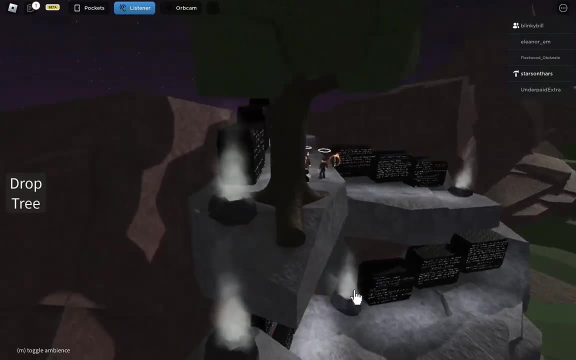 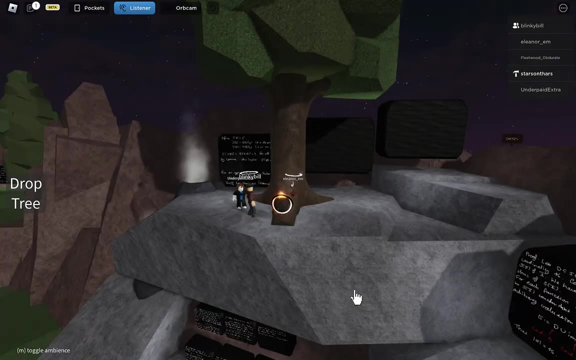 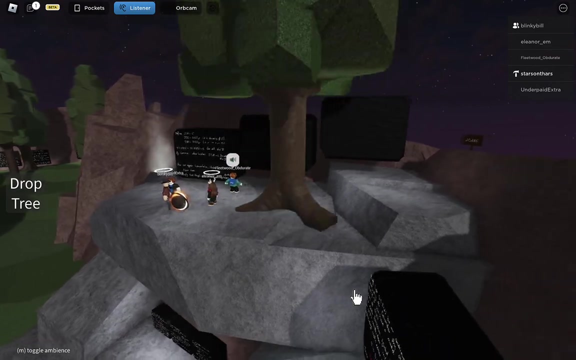 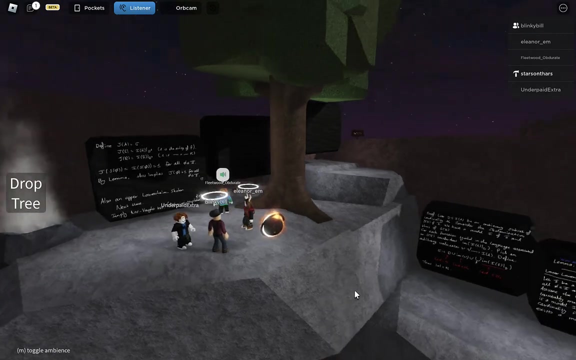 I think there's a lot of them. I think that the fact that you can write first order formulas not in- I'm getting distracted by the nature- the fact that you can write formulas not in pre-next normal form, for example, is what I mean by redundancy. But why do we have formulas? 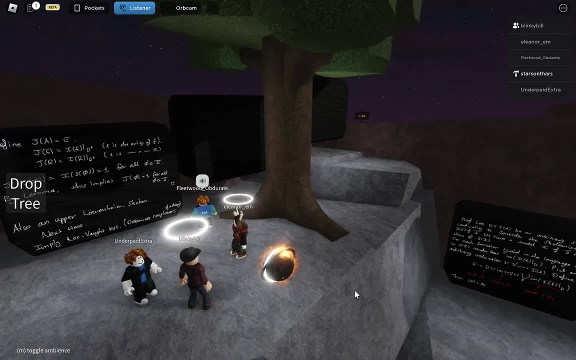 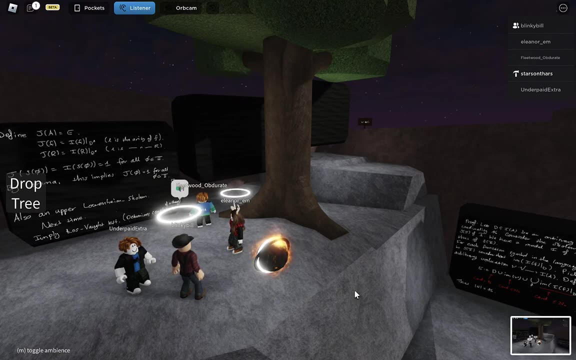 that aren't in pre-next normal form. Yeah, Yeah, I don't really get your point there. Could you speak more to that? Okay, so let's think about the injection of, like natural deduction into proofnets or something. That's where these ideas really come from. in my opinion, Proofnets are very-. 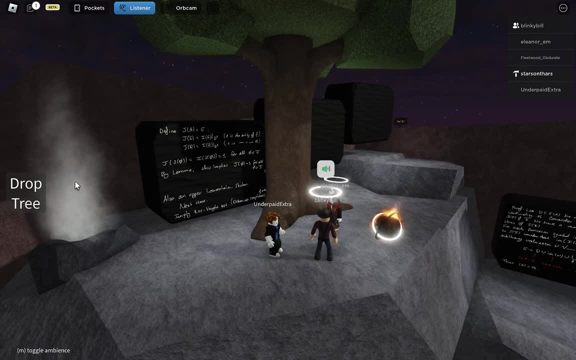 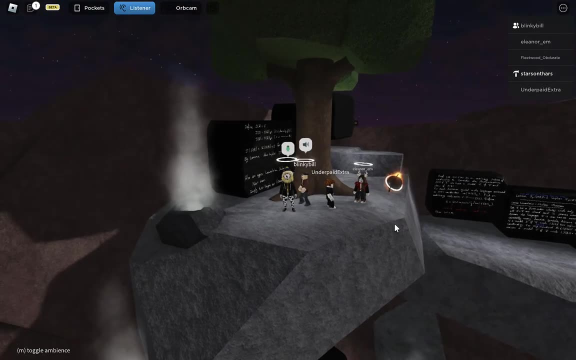 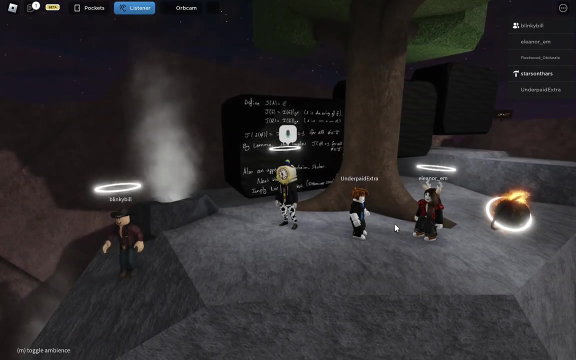 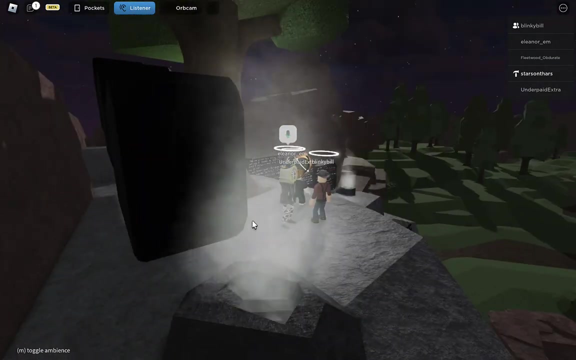 See ya, Did you just yeet Will into pain? Oops, Okay, that was bad form. I was planning to stand on his head and then let go of the tree, so he possessed it unwillingly. That was my aim. Where did he end up? 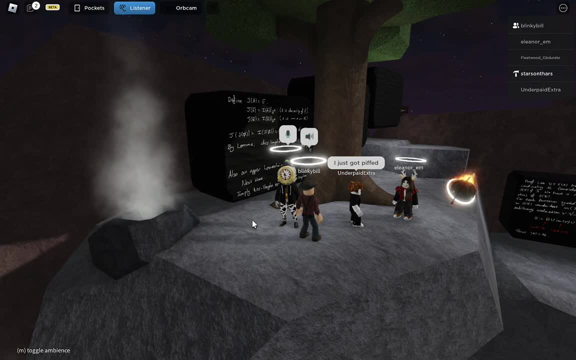 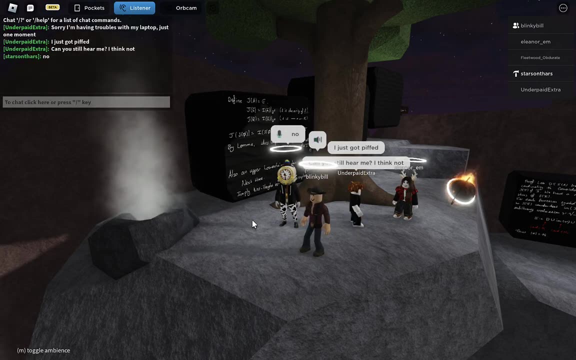 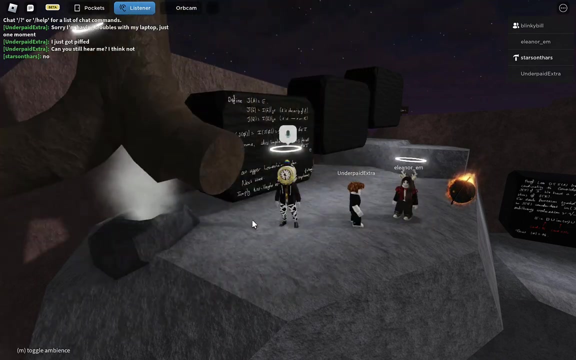 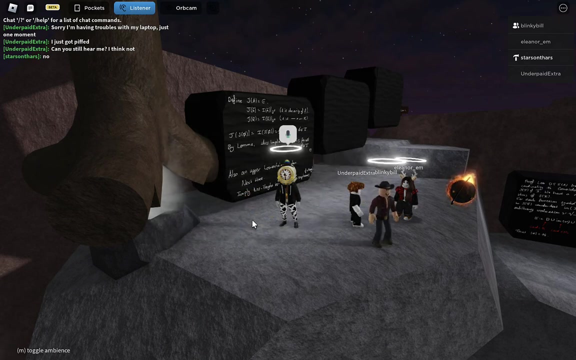 I don't know, He should come down at some point. Yeah, we can't hate him. Yeah, we can't hate him, Okay, Okay then. Oh my God, How could you? Yeah, that's pretty bad. He was mid-sentence too. 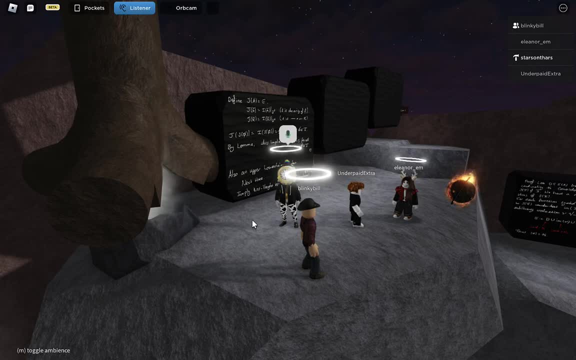 Oh well, He'll come back enlightened by his journey through the cosmic Spaces 270?? Yeah, might have been so high into the air that he actually exceeded the the like boundary from above, like there's a boundary which it just starts destroying parts. 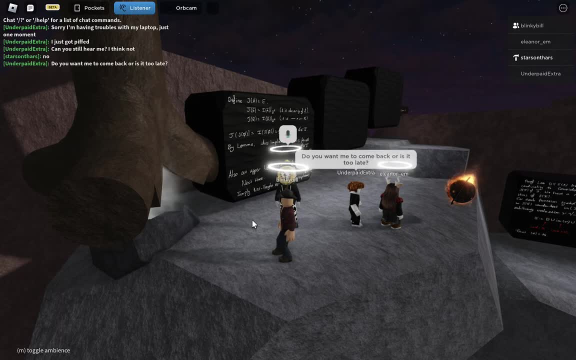 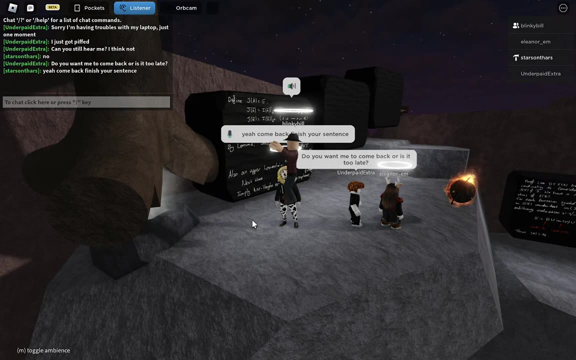 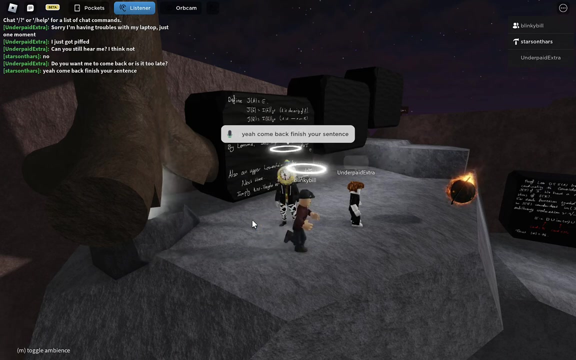 well, you didn't, you didn't reset, he quit. i am gonna go. you'll have a good night. okay, see, ya, see y'all. thanks for coming. um, yeah, uh, well, i was expecting him to fall back down. at least i don't know what happened. thank you, donkey. 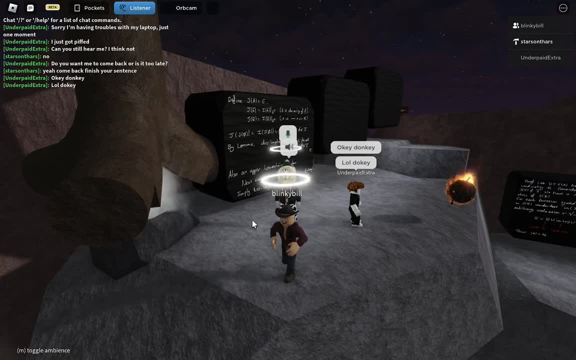 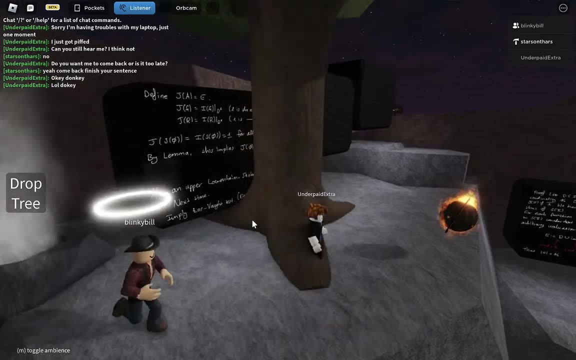 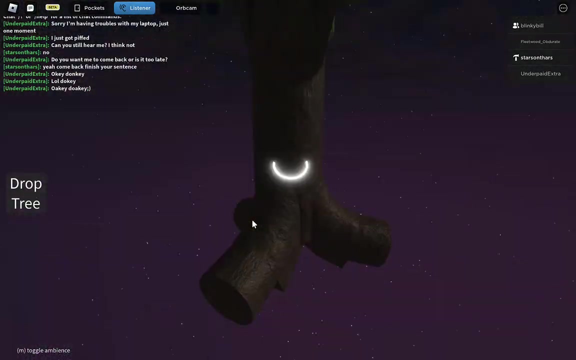 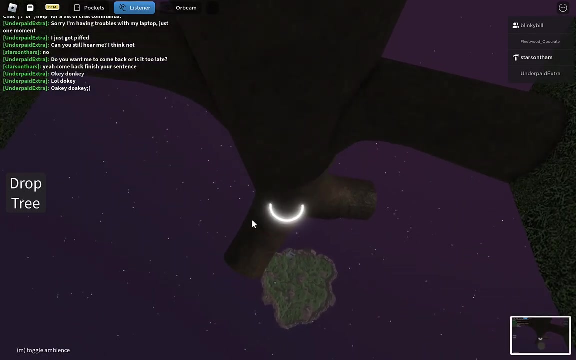 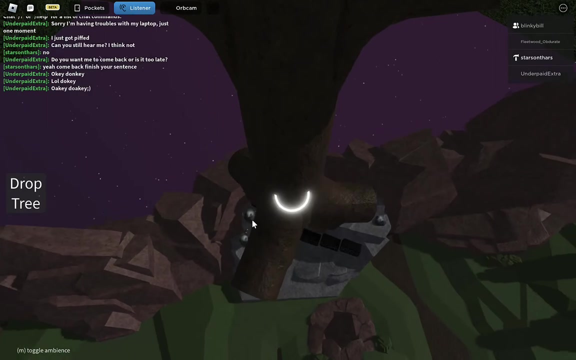 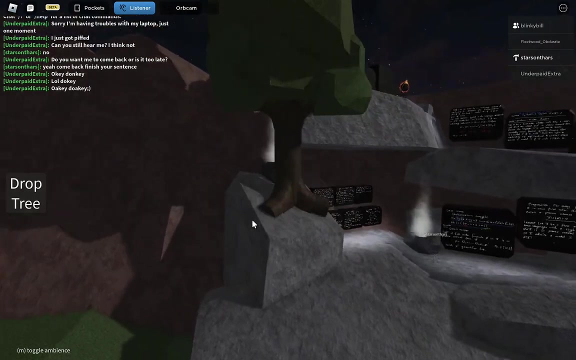 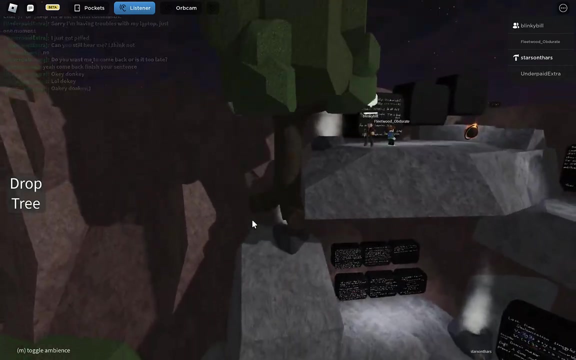 you might as well do something productive and eat his other. oh what? oh no, what was that doof he just sent himself? can you hear me? yeah, that was that was interesting. okay, can you hear me? yeah, i can hear you. did you see what happened to dan just then? 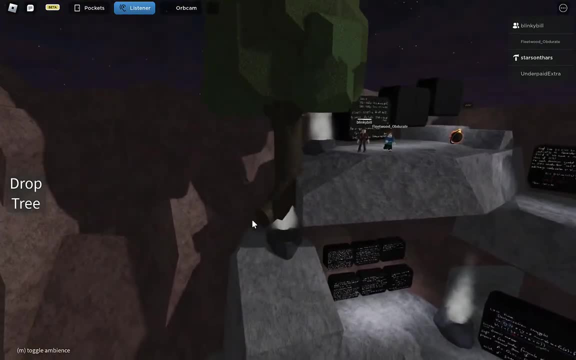 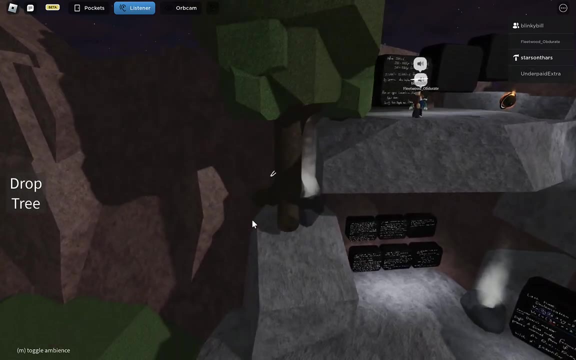 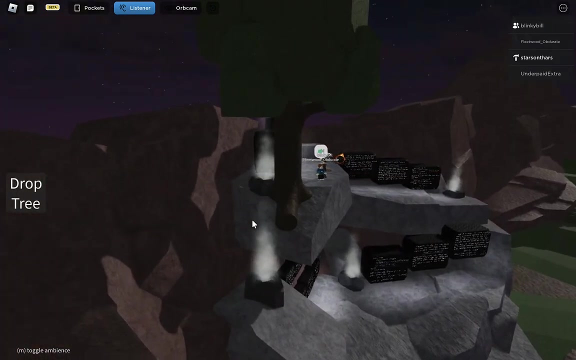 what did you do? no, what happened? i went flying up where you were. well, he like, yeah, i got completely piffed. it was really quite funny. did you go like so high in the sky? it like killed you. i have no idea where i went, but i was rotating at an incredible rate. 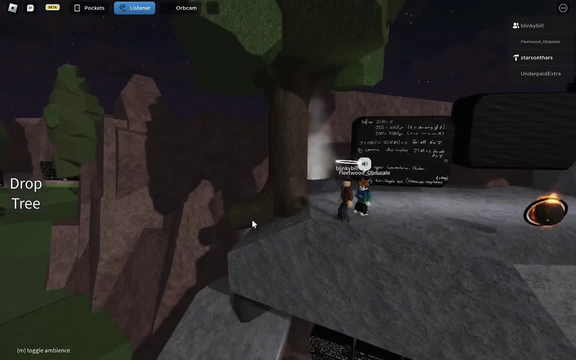 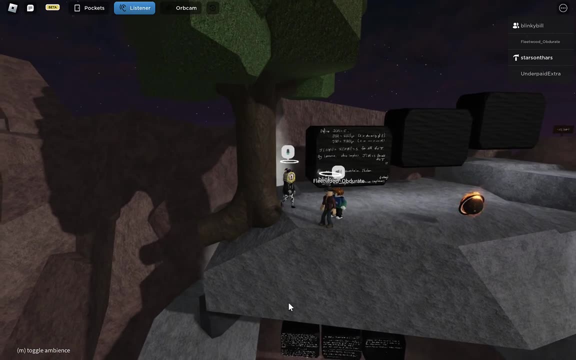 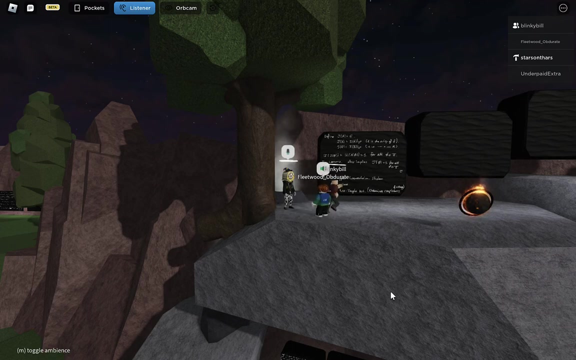 and i was in the middle of nowhere. i didn't die, but i was definitely launched. ah, so you didn't kill anybody, yeah, okay, let me finish my sentence now. this is something that i haven't fully made up my mind about, but i think that there's an interesting observation to be made. proof nets are kind of 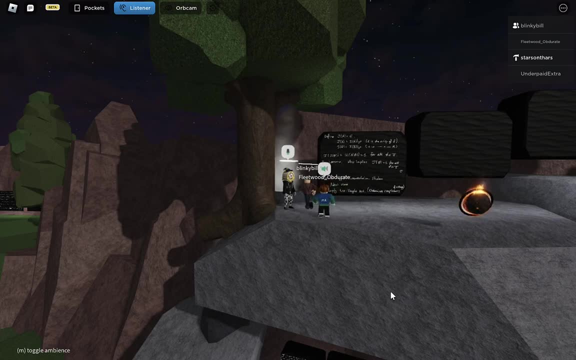 interesting because they move away a lot of the different ways that they're being moved around the area. because they're moving away a lot of the different ways that they're being moved around, the different ways that you can write what is quote-unquote: the same proof, right, and this is a. 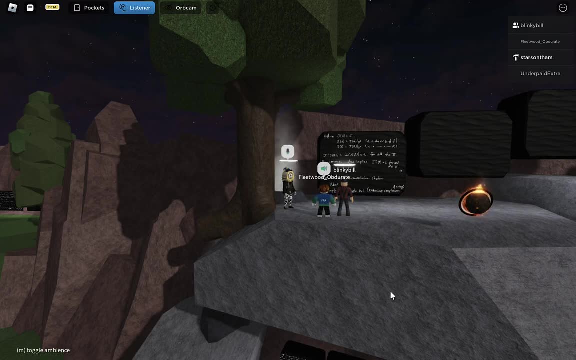 common complaint over systems, for example the intuitionistic second calculus. you've got all of these different commutation rules that need to be modded out before you get the same lambda term inside there, against the duality, for example. so the same quote-unquote proof is written out in a 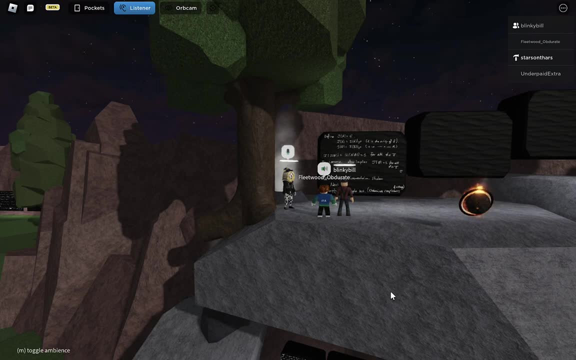 billion different ways, but proof nets only have one way to write out the same proof. you know if you distinguish cut equivalents, and what's interesting about that is it reveals mathematical structure, for example the sequentialization theorem or the cut elimination theorem, i suppose. but let's go with the sequentialization theorem. that also holds for intuitionistic proofs in some. 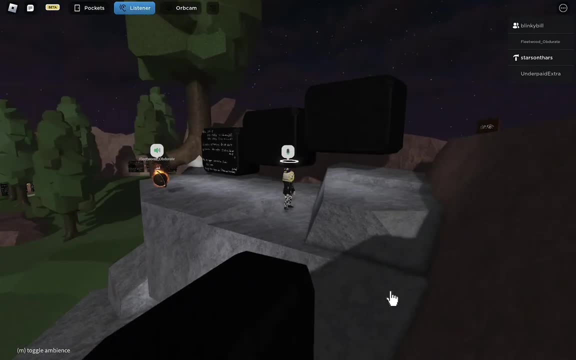 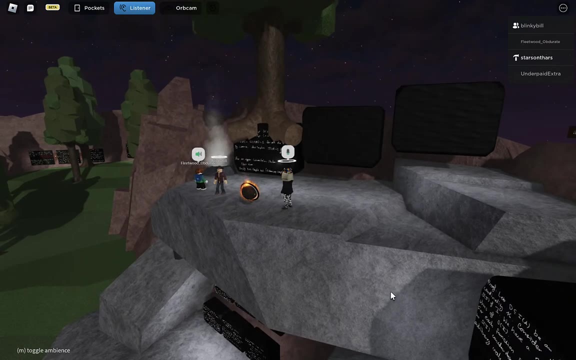 sense, but it's much more difficult to observe and to see because your notation is cumbersome. you've got redundancy inside your notation, okay. now, sometimes that redundancy is in fact a positive thing, though. for example, in the lambda calculus you also have that redundancy if you distinguish alpha equivalent terms. so you've got all of these different ways of writing. 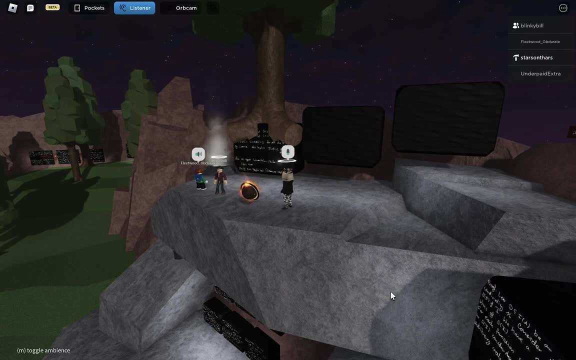 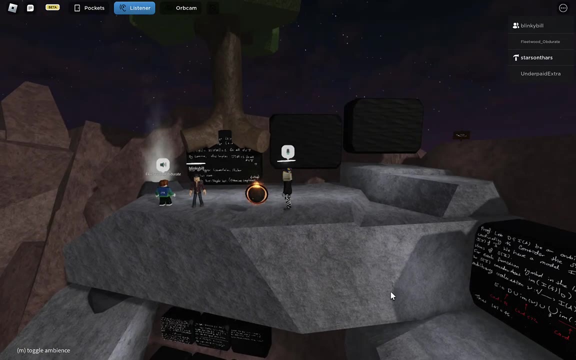 out quote-unquote the same term, right, but that's kind of, in fact, beneficial, if you, because the reason why it's beneficial is because people have defined lambda calculus systems where the alpha equivalence is not visible inside the notation, and it comes down to really awful things. 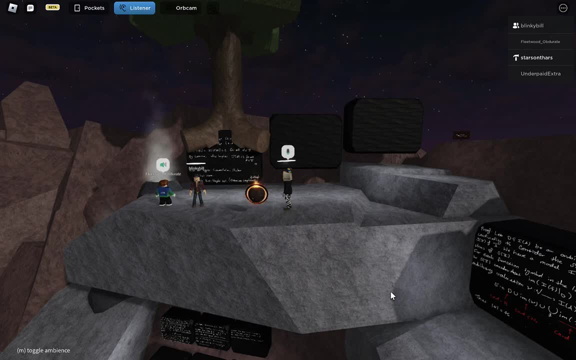 like bracket counting and stuff like that. so a computer would be able to distinguish the terms very easily, but a human would struggle to, and so the alpha equivalence in fact makes it easier to read, even though it's redundant. but that makes sense anyway. redundancy increases simplicity of. 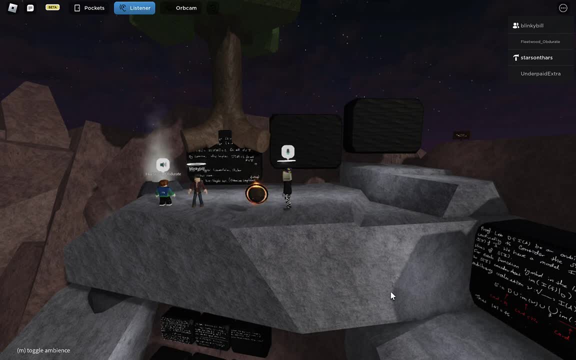 you know reading it, there are many different ways to read the same thing. okay, but this fact about the proof nets being eloquent in that they only give you one way to write out the same proof is really interesting to me, because i think that when you have less redundancy in notation, you 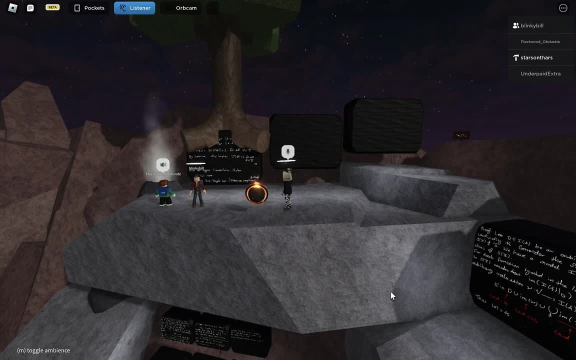 have a higher chance of revealing mathematical structure. so i think that first order logic is very interesting because it seems to be very close to the way that we as humans ever could possibly reason. but when you do anything with the system you realize that there's a lot of redundancy. 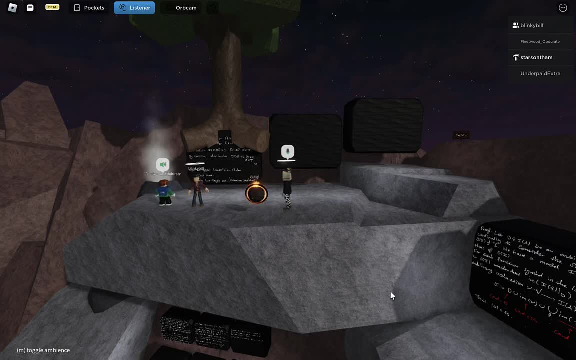 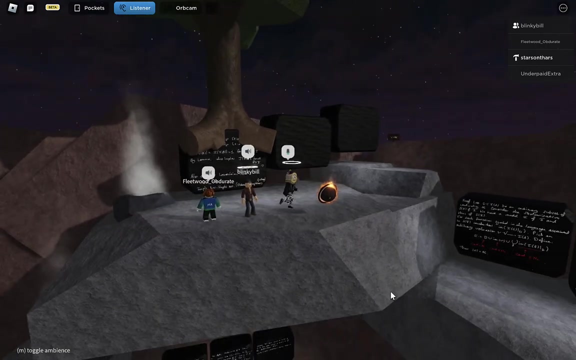 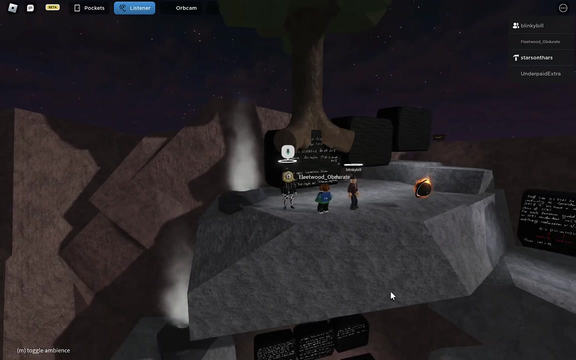 and a lot of tedium involved in working with it. so i wonder if there's a more elegant system that does away with all of that redundancy, which might reveal more mathematical structure, for instance? yeah, i mean, you're skating close to topics that are related to statistical learning. uh, there are key advantages to redundancy. 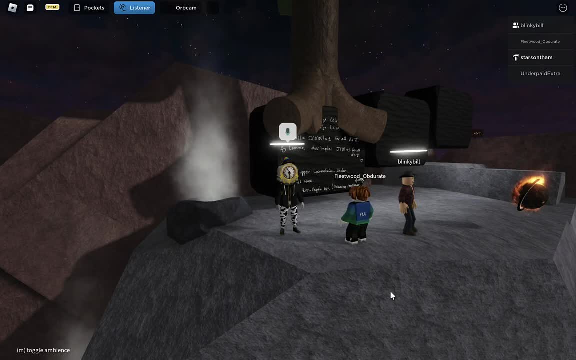 that come from. well, exactly the things you're talking about. you can make some of that formal, so i think that's a good point. i think that's a good point. i think that's a good point. i think i would speculate that there is a there's a limit to how much redundancy you can eliminate without 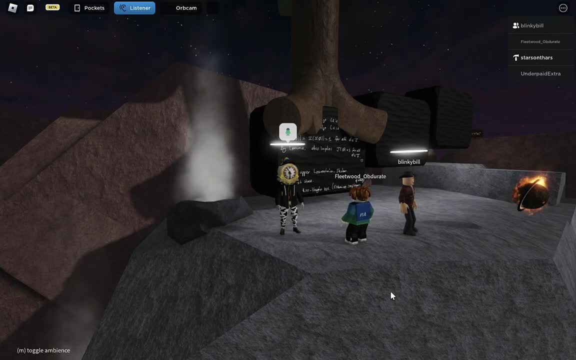 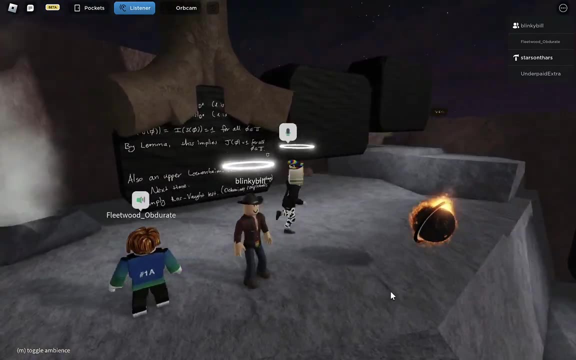 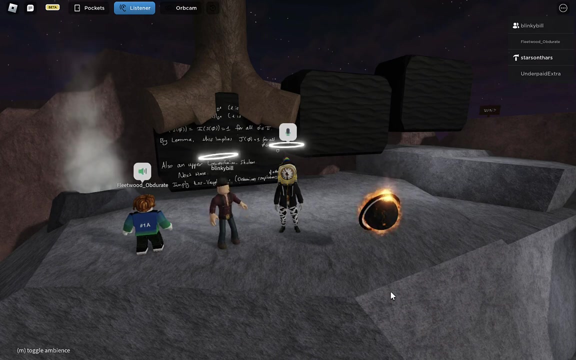 making it very difficult for finite learning systems to actually find those terms or proofs so interesting. yeah, yeah, you can literally say that with a lambda calculus like: go and have a look at these notations for the lambda calculus that don't have alpha equivalents inside them, and that's literally the problem that you run into. yeah, so it doesn't surprise me. that's really.